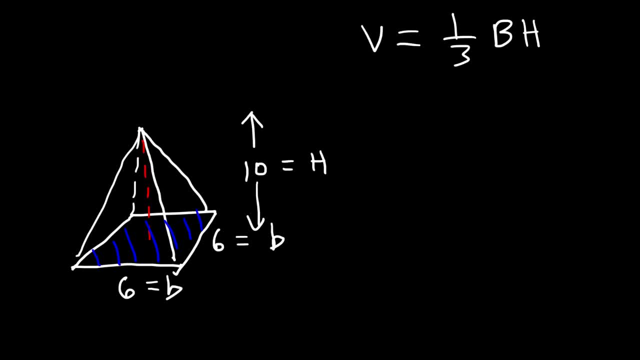 You can call it s or x if you want to, depending on if that's the way your teacher taught it or if it's in your textbook, like that. But I'm going to use lowercase b for the side length of the base and capital B for the area of the base. 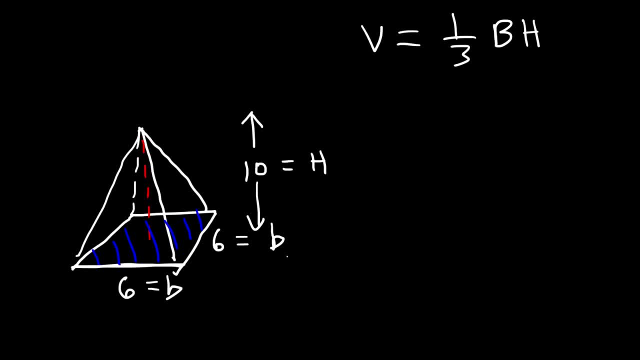 So to find the area of the square, it's going to be the length times the width, or simply b squared. So the area of the base is b squared. So therefore, the volume of this entire square-based pyramid is 1 third times the side length squared, multiplied by the height of the pyramid. 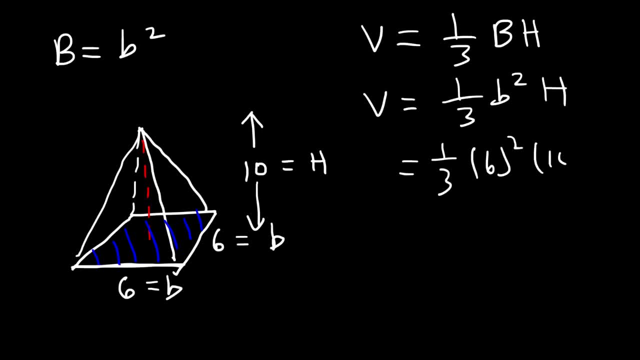 So it's going to be 1 third 6 squared times 10.. 6 times 6 is 36.. And 1 third of 3.. 36 or 36 divided by 3, that's 12.. And 12 times 10 is 120.. 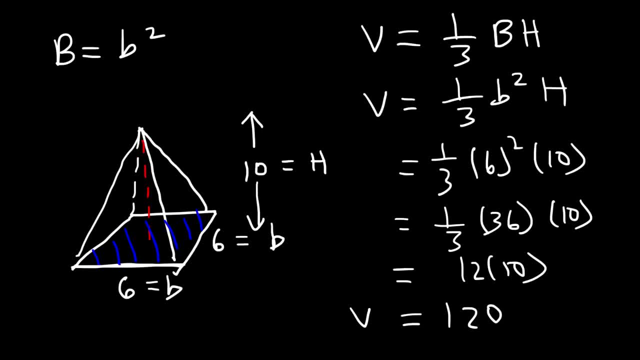 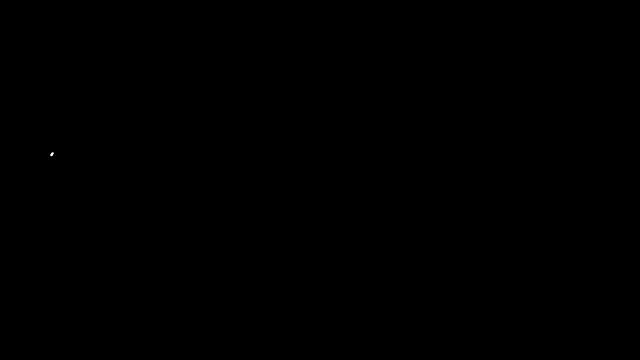 So the volume is 120 cubic units. So let's say if this was 6 inches, the volume would be 120 cubic inches if everything was in inches. Let's try another practice problem. So go ahead and find the volume of this pyramid. 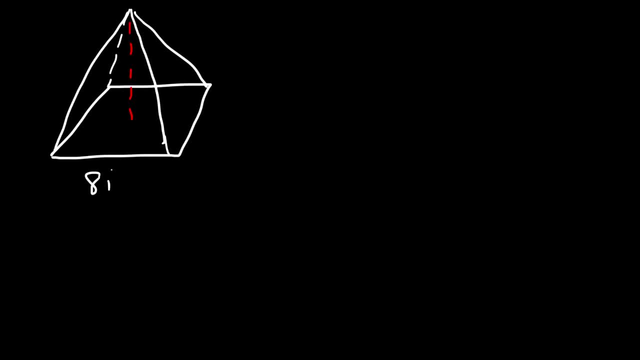 So let's say the side lengths are 8 inches And the height, let's say it's 12 inches. So feel free to pause the video and find the volume of this pyramid. So the volume is going to be 1 third times the area of the base multiplied by the height of the pyramid. 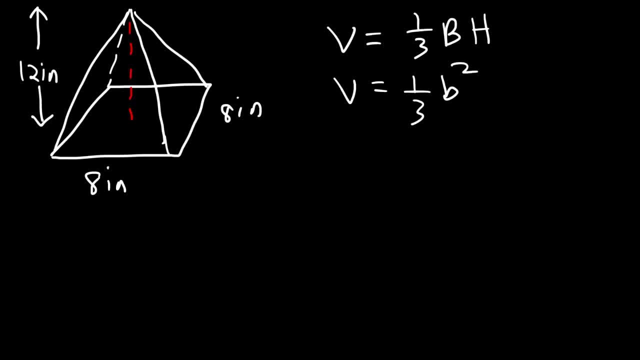 And the area of the base, as we defined in the last example, is going to be the side length of the square squared. So basically just b squared. So now example b: lowercase b is 8, and the height is 12.. 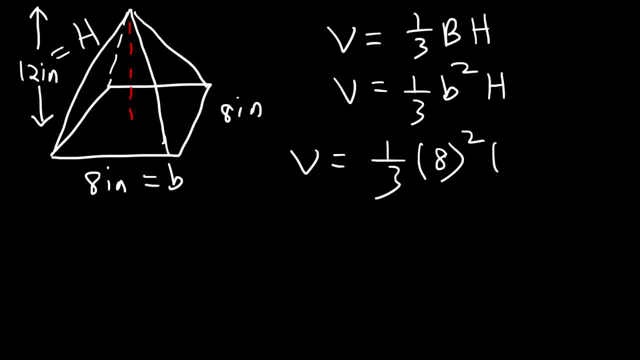 So it's 1 third multiplied by 8 squared times 12.. 1 third of 12, or 12 divided by 3, that's 4.. And 8 squared is 64.. 4 times 64 is 256.. 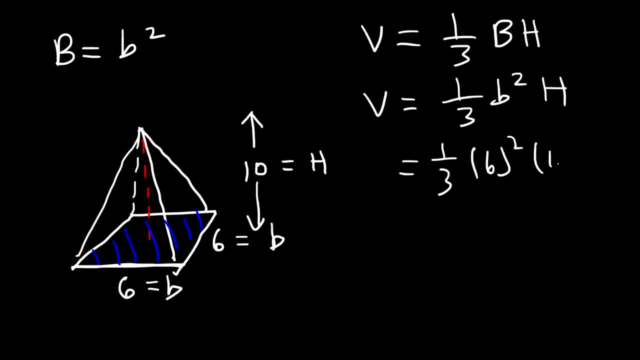 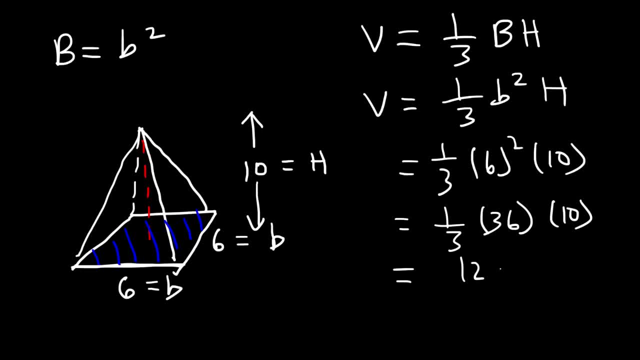 And 1 third of 36 is 36.. And 1 third of 36, or 36, divided by 3, that's 12.. And 12 times 10 is 120. So the volume is 120 cubic units. So let's say if this was 6 inches, the volume would be 120 cubic inches. if everything was in inches. 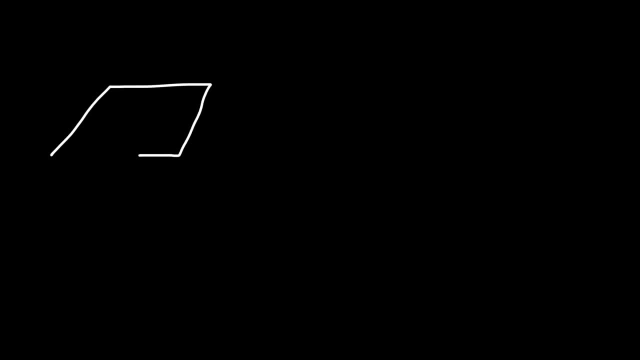 Let's try another practice problem. So go ahead and find the volume of this pyramid. So let's say the side lengths are 8 inches And the height, let's say it's 12 inches. So feel free to pause the video and find the volume of this pyramid. 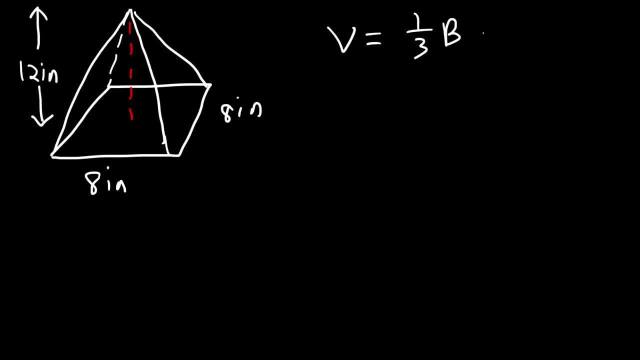 So the volume is going to be 1 third times the area of the base, multiplied by the height of the pyramid. And the area of the base as we defined in the last example is going to be the side length of the square squared. 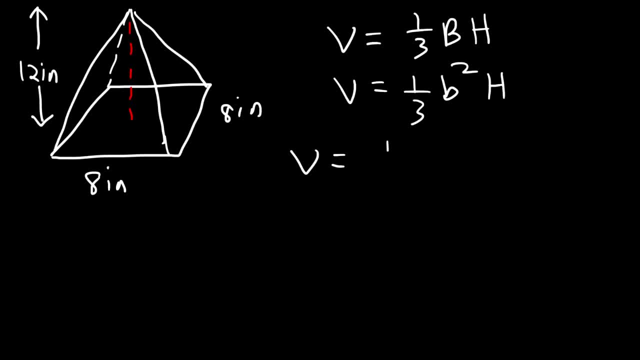 So basically just b squared. So now example b: lowercase b is 8, and the height is 12.. So it's 1 third multiplied by 8 squared times 12.. 1 third of 12, or 12 divided by 3,, that's 4.. 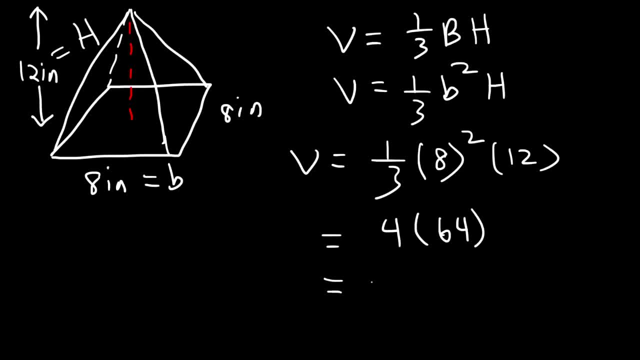 And 8 squared is 64.. 4 times 64 is 256.. So the volume is 256 cubic inches, And so that's the answer for this example. Now let's talk about finding the slant height of a square-based pyramid. 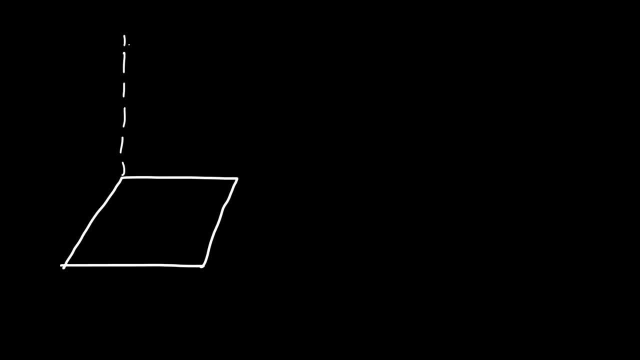 So let me just draw this first. I want to draw this carefully Now. the red line is the height of the pyramid, as we talked about before. So this makes a right angle with the plane And this makes a left angle with the plane, as we talked about before. 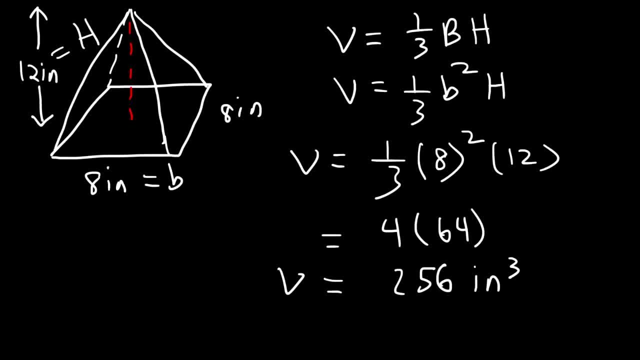 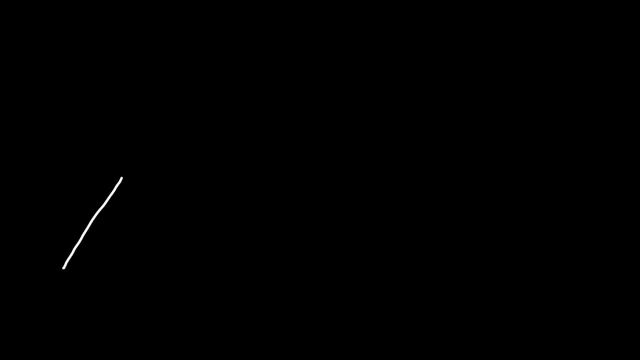 So the volume is 256 cubic inches, And so that's the answer for this example. Now let's talk about finding the slant height of a square-based pyramid. So let me just draw this first. I want to draw this carefully. 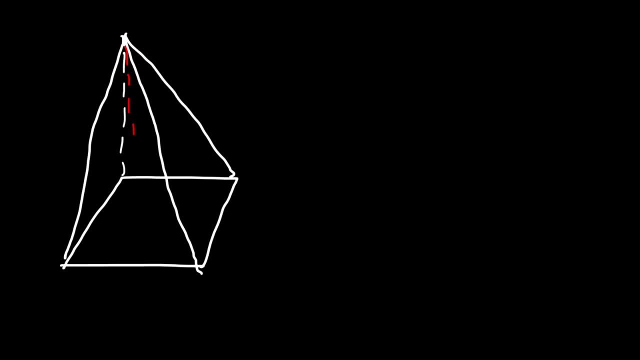 Now, the red line is the height of the pyramid, as we talked about before, So this makes a right angle with the plane And this is the height of the pyramid. The line in green is the slant height, So make sure you're aware of the difference between these two. 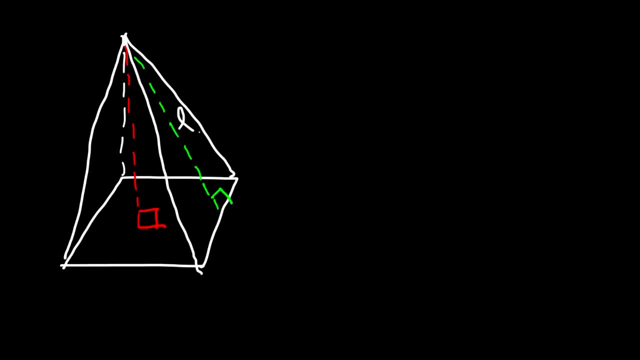 So this is L, which represents the length of the green dashed line, And the red dashed line that represents the height of the pyramid. We're going to say b represents the side length of the square. Now we've talked about the volume of the pyramid. 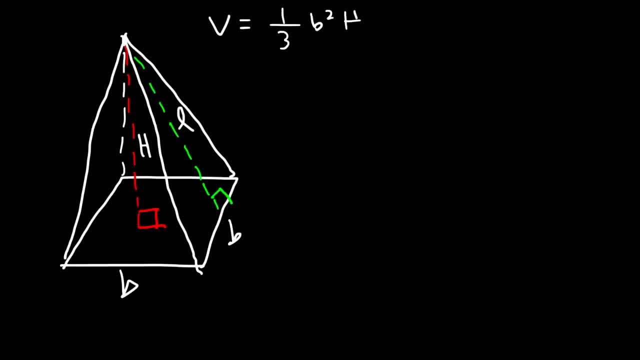 It's 1 third b squared times h, or 1 third the area of the base times h. But now if you want to find a surface area, you need to use the slant height instead of the actual height. The surface area is the area of the base plus the lateral area. 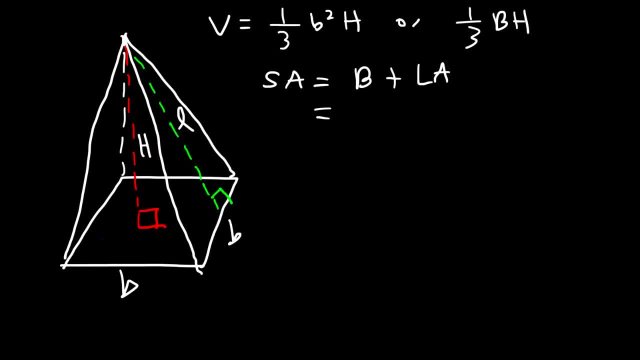 Now the area of the base is simply the area shaded in blue, And basically that's just b squared. Now what about the lateral area? Notice that this pyramid has four triangles. Here's one of the triangles shaded in blue. 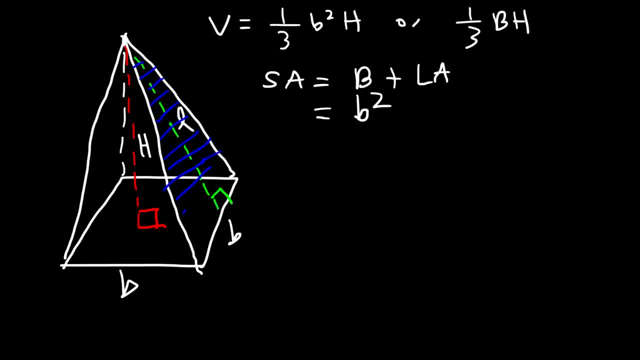 So that's the triangle on the right side. You have a triangle on the left, one in the back and one in the front, So that triangle. I'm just going to redraw it, Just a side view. So this is the base length of the square, which is also the base of the triangle. 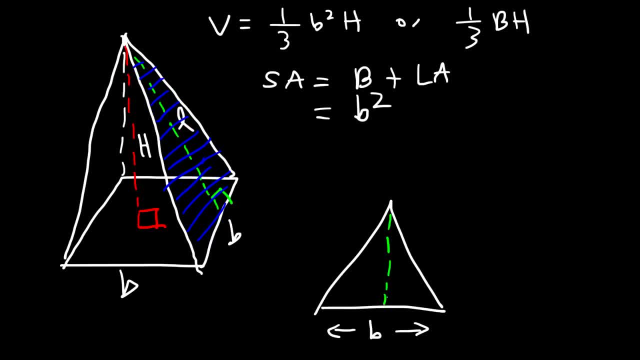 And the line in green represents the slant height of the triangle, which is l. Now, whenever you have a triangle, if you know the base and if you know the height of the triangle, to find the area is simply 1 half base times height. 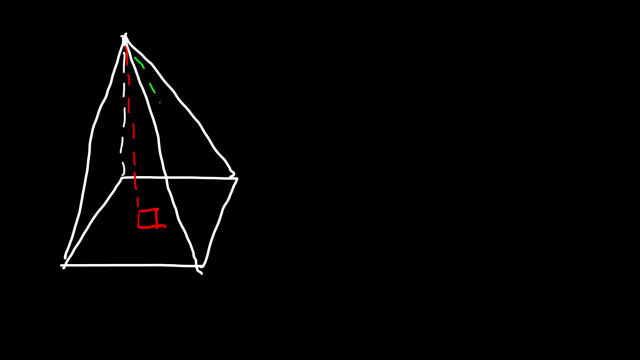 And this makes a right angle with the plane, as we talked about before. The line in green is the slant height, So make sure you're aware of the difference between these two. So this is L, which represents the length of the green dashed line, and the red dashed line that represents the height of the pyramid. 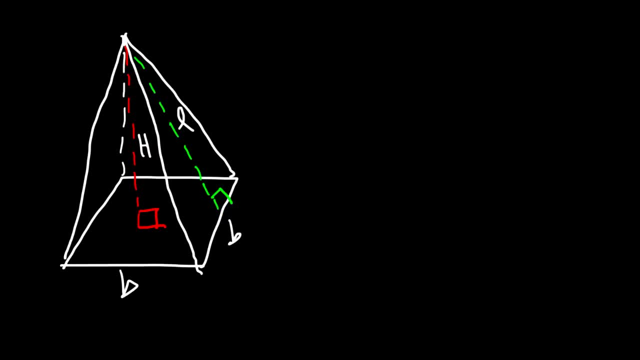 We're going to say b represents the side length of the square. Now we've talked about the volume of the pyramid. It's 1 third b squared times h, or 1 third the area of the base times h. But now, if you want to find a surface area, you need to use the slant height instead of the actual height. 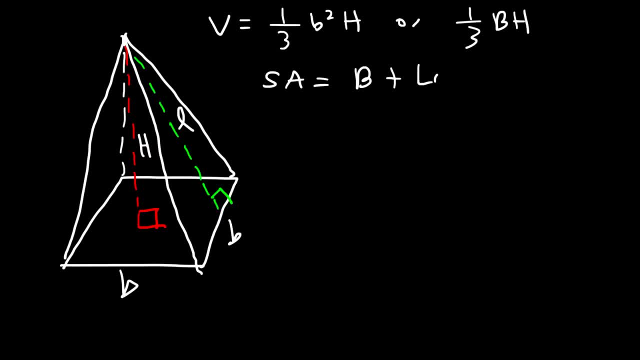 The surface area is the area of the base plus the lateral area. Now, the area of the base is simply the area shaded in blue, And basically that's just b squared. Now what about the lateral area? Notice that this pyramid has four triangles. 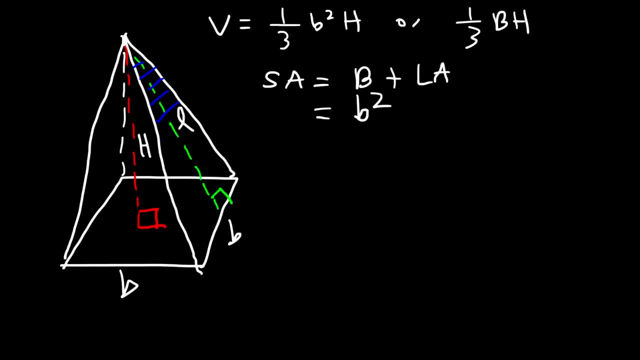 Here's one of the triangles shaded in blue. So that's the triangle on the right side. You have a triangle on the left, one in the back and one in the front, So that triangle I'm just going to redraw. 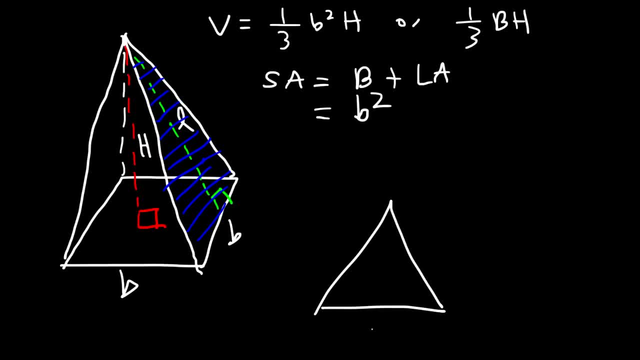 Just a side view of it. So this is the base length of the square, which is also the base of the triangle, And the line in green represents the slant height of the triangle, which is l. Now, whenever you have a triangle, if you know the base and if you know the height of the triangle, 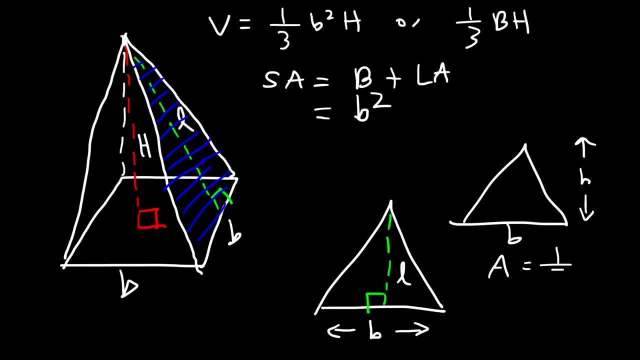 to find. the area is simply 1 half base times height, But in this case the height is the slant height, So the area becomes 1.5.. The area becomes 1.5 base times slant height, which is l. 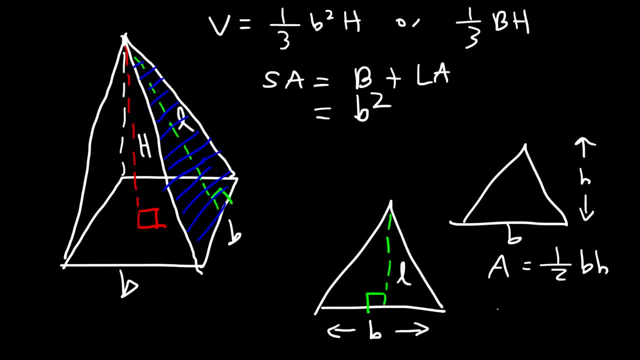 But in this case the height is the slant height, So the area becomes 1 half base times slant height, which is l. Now the triangular pyramid has four triangles. You have one on the left, highlighted in green. 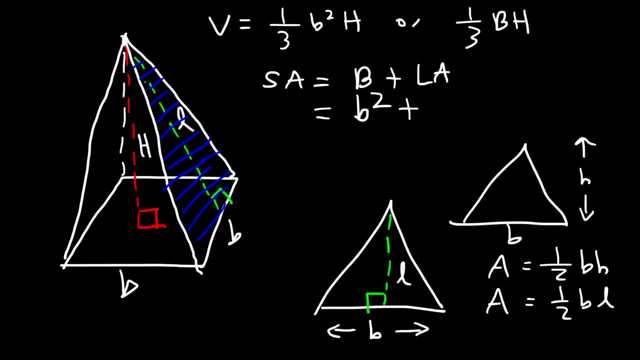 And then you have one in the back which is The blue line's kind of overlapping it, but you can see it in the back there, And then the one in the front represented by the portion shaded in yellow. So therefore it's going to be 4 times the area of each of those triangles, which is 1 half b times l. 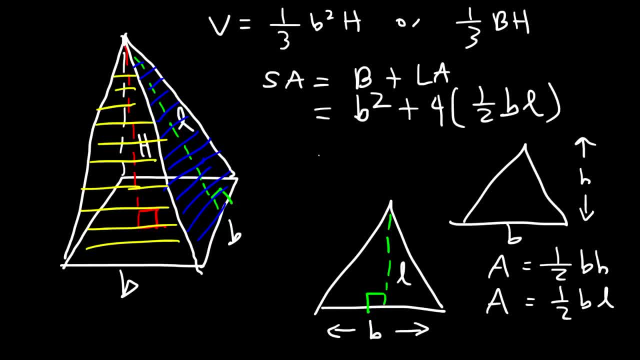 So 4 times the half is 2.. So therefore, the surface area. you can find it using this equation. It's b times l, So that's the formula I'm going to use to find the surface area of a square base pyramid. 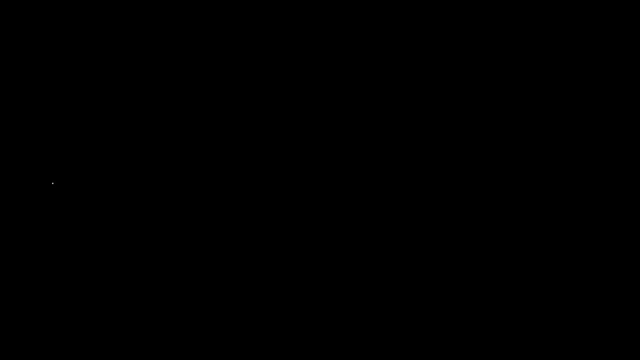 It's the area of the base plus the lateral area. Go ahead and try this example. So let's say, if you're given the slant height, And let's say it's 15 centimeters, And you're given the length of the base, 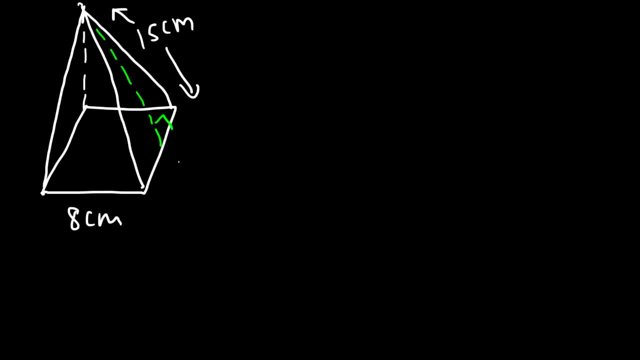 Let's say it's 8 centimeters, It's 8 by 8.. Go ahead and calculate the surface area of this Object or figure And also find the lateral area as well. Now, the first thing I would do is find the lateral area. 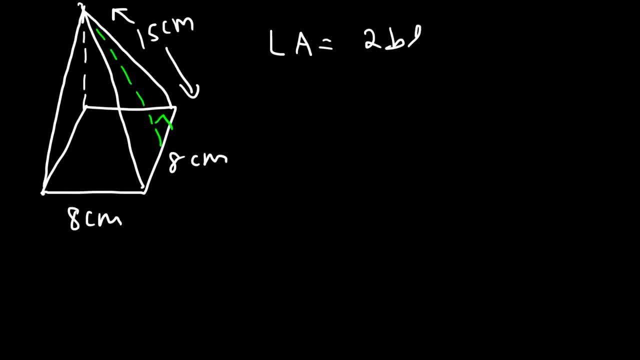 The lateral area is simply 2bl. As you mentioned before, it's 1 half base times height, Or, in this case, slant height. That's the area of each triangle And there's 4 triangles, so times 4.. 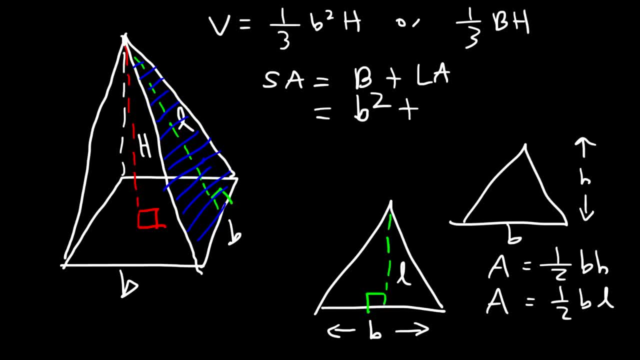 Now the triangular pyramid has four triangles. You have one on the left, highlighted in green, And then you have one in the back which is The blue line's kind of overlapping it, but you can see it in the back there. 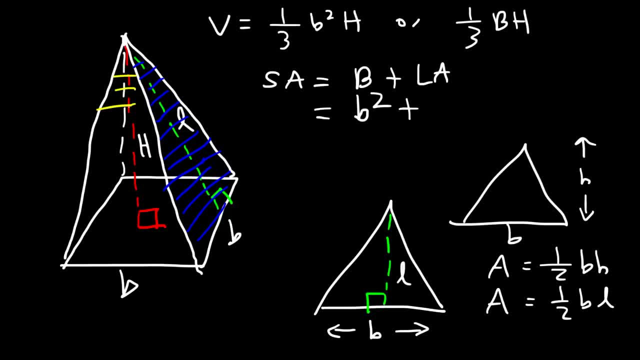 And then the one in the front represented by the portion shaded in yellow. So therefore it's going to be 4 times the area of each of those triangles, which is 1 half b times l. So 4 times 1 half is 2.. 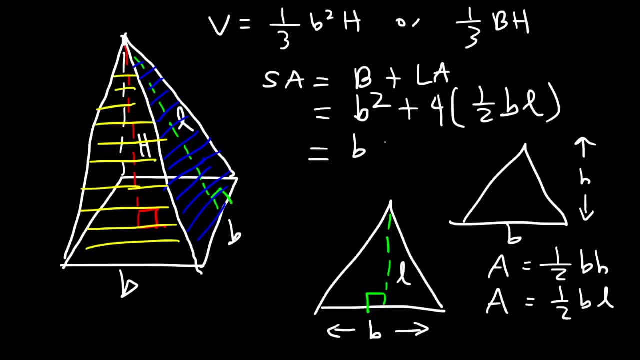 So therefore, the surface area. you could find it using this equation: It's b squared plus 4. I mean 2bl. So that's the formula I'm going to use to find the surface area of a square base pyramid. 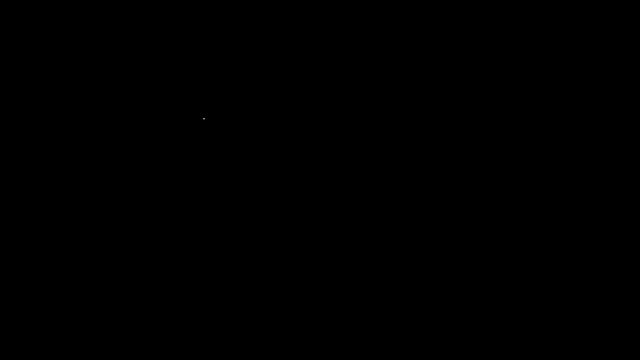 It's the area of the base plus the lateral area. Go ahead and try this example. So let's say, if you're given the slant height, And let's say it's 15 centimeters, And you're given the length of the base, 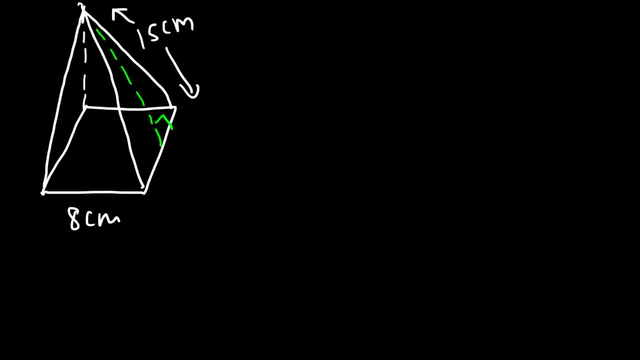 Let's say it's 8 centimeters, It's 8 by 8. Go ahead and calculate the surface area of this object or figure And also find the lateral area as well. Now, the first thing I would do is find the lateral area. 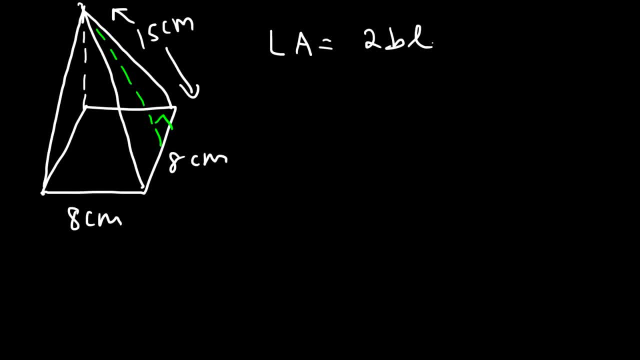 The lateral area is simply 2bl. As we mentioned before, it's 1 half base times height or, in this case, slant height. That's the area of each triangle, And there's 4 triangles, so times 4.. 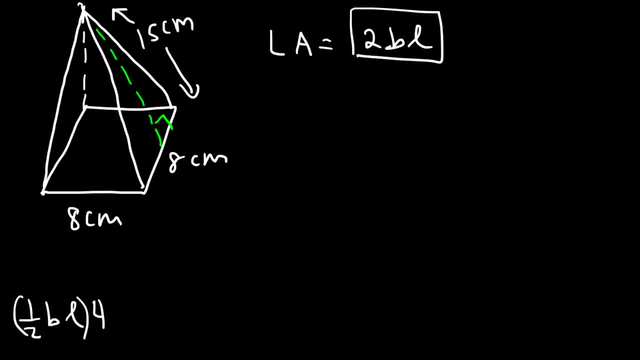 And that gives us 2bl. So that will give you the lateral area, The area of the 4 triangles. So b in our example is 8. And l is 15.. So it's 2 times 8 times 15.. 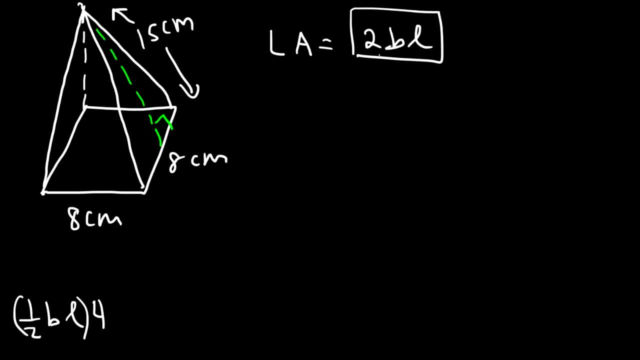 And that gives us 2bl. So that will give you the lateral area, The area of the 4 triangles. So b in our example is 8. And l is 15.. So it's 2 times 8 times 15.. 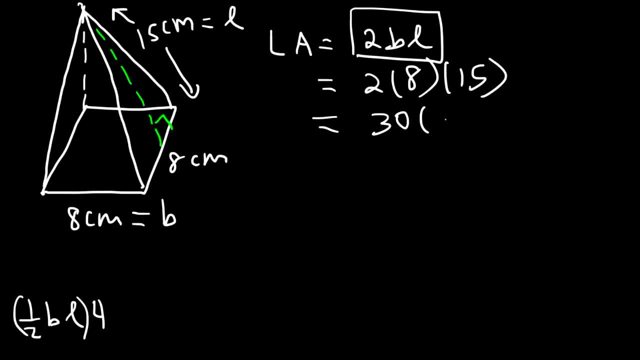 Now, 2 times 15 is 30. And 30 times 8.. If 3 times 8 is 24,, 30 times 8 is 240.. So it's 240 square centimeters. So that's the lateral area. 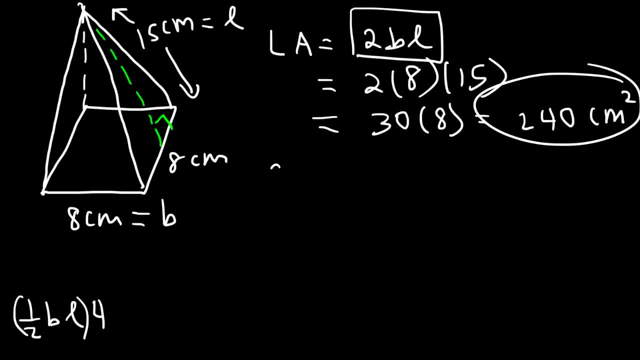 Now what we need to do next is we need to find the surface area. It's the area of the base plus the lateral area, So it's going to be b squared plus 2bl b squared, that's going to be 8 squared. 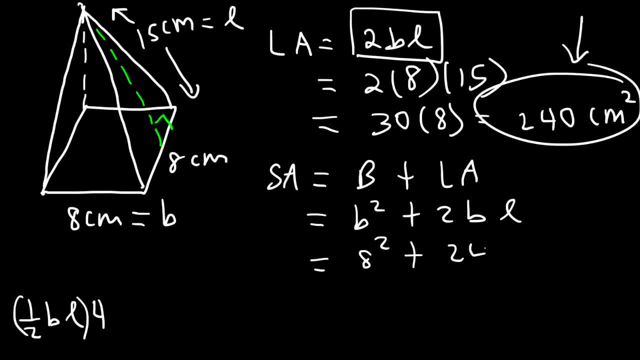 And 2bl is 240.. 8 squared is 64.. 64 plus 240, that's going to be 304.. So the surface area is 304.. So it's going to be 304 square centimeters. And so now you know how to find the surface area and the lateral area of a square-based pyramid. 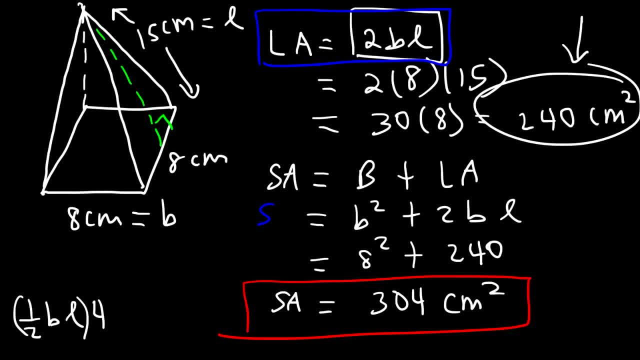 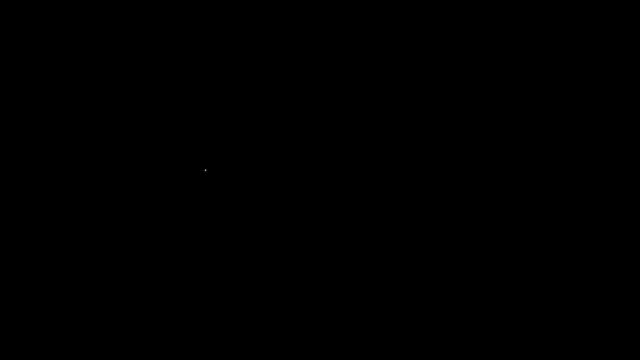 So these are the two equations that you need. Now let's work on another problem. Let's say the height is 12 inches, So that's going to be the height of the pyramid. And let's say the base is 10 inches long and 10 inches wide. 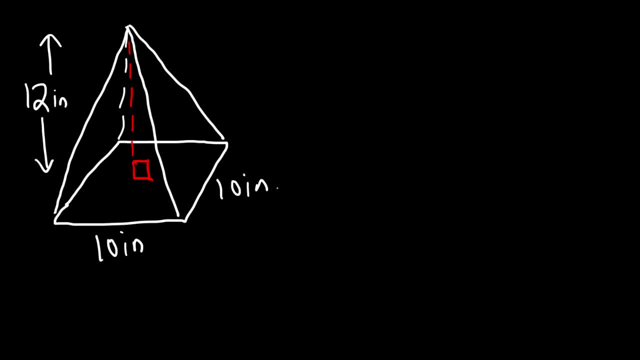 So, using this information, find both the volume and the surface area of this pyramid. So be careful with this problem. So go ahead and take a minute and work on this problem. Feel free to pause the video too. So let's start with the volume. 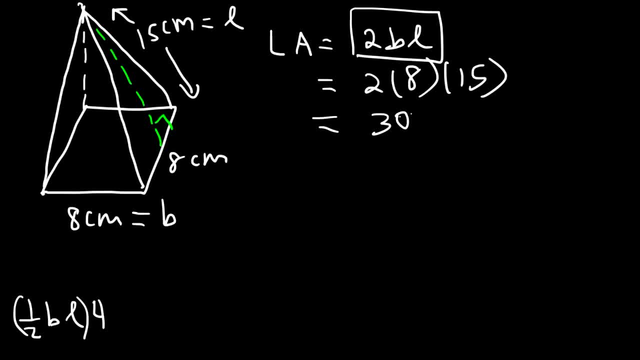 Now, 2 times 15 is 30. And 30 times 8.. If 3 times 8 is 24,, 30 times 8 is 240.. So it's 240 square centimeters. So that's the lateral area. 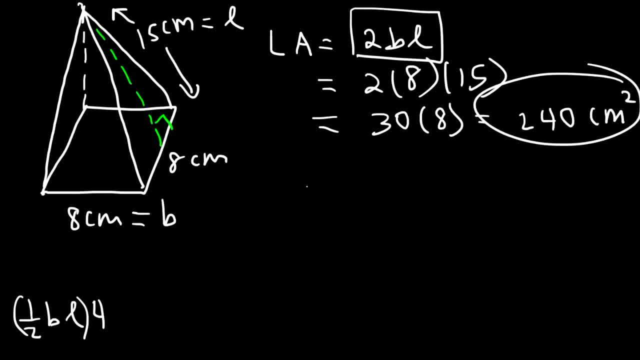 Now what we need to do next is we need to find the surface area. It's the area of the base plus the lateral area, So it's going to be b squared plus 2bl b squared, that's going to be 8 squared. 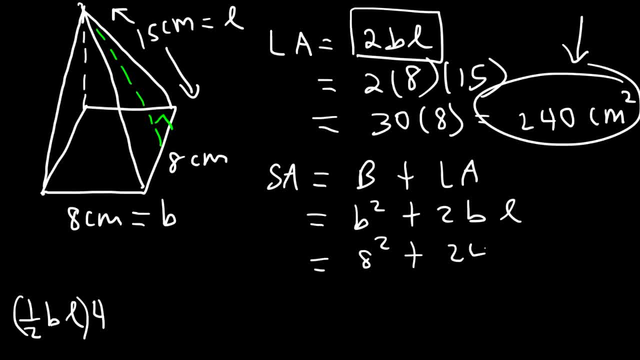 And 2bl is 240.. 8 squared is 64.. 64 plus 240, that's going to be 304.. So the surface area is 304 square centimeters, And so now you know how to find the surface area. 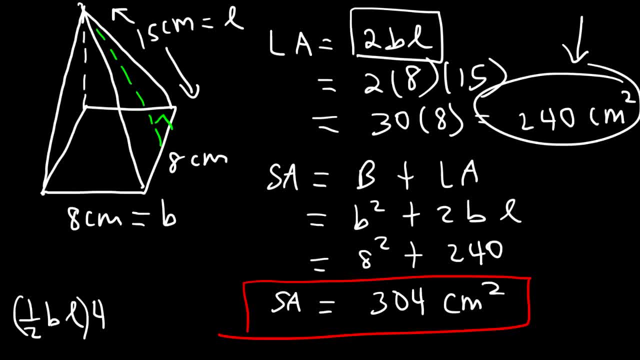 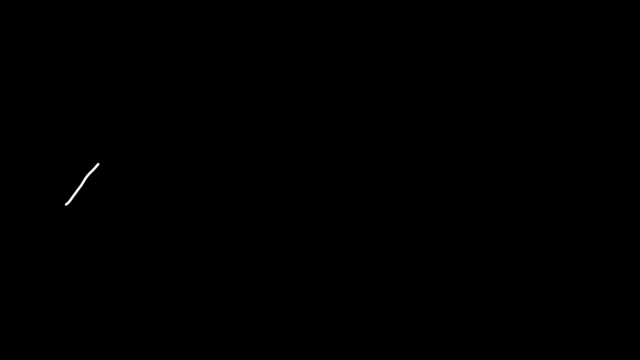 and the lateral area of a square-based pyramid. So these are the two equations that you need. Now let's work on another problem. Let's say the height. Let's say the height is 12 inches, So that's going to be the height of the pyramid. 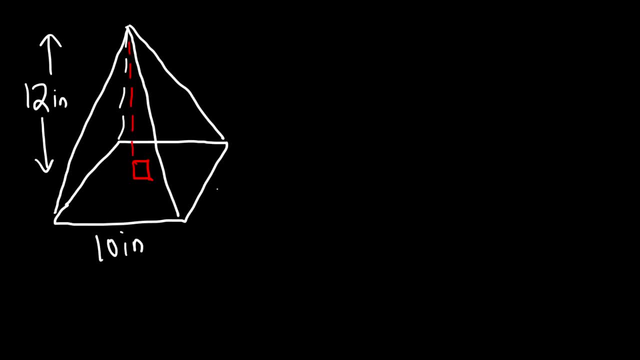 And let's say the base is 10 inches long and 10 inches wide. So, using this information, find both the volume and the surface area of this pyramid. So be careful with this problem. So go ahead and take a minute and work on this problem. 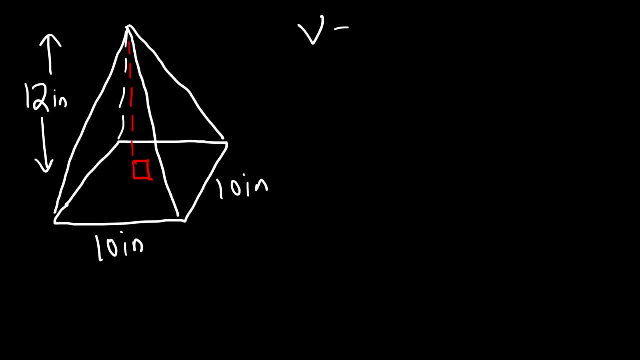 Feel free to pause the video too, So let's start with the volume. It's 1 third base times height, Which is 1 third. the side length squared times the height of the pyramid B is 10. And the height is: 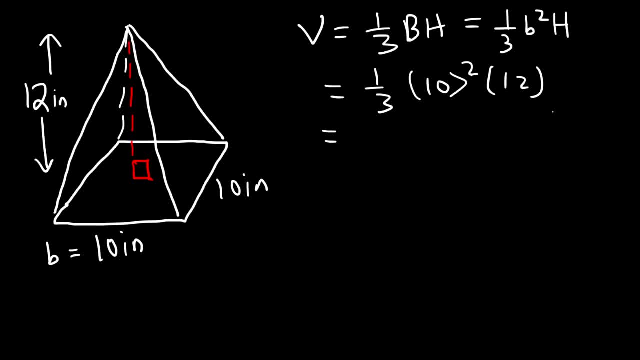 12.. So 1 third of 12 is 4. And 10 squared is 100.. So in this problem the volume is 400 cubic inches. So that wasn't bad. Now what about the surface area And also the lateral area? 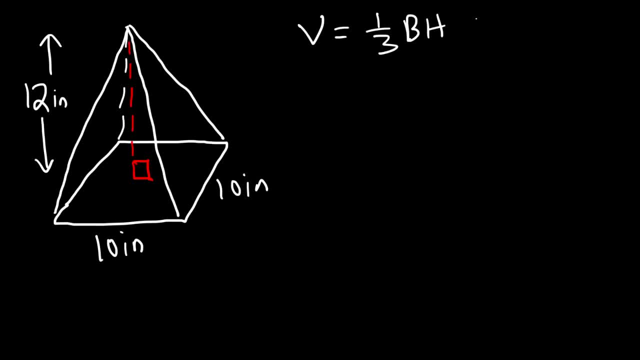 It's 1 third base times height, which is 1 third the side length squared times the height of the pyramid. b squared b is 10.. And the height is 12.. So 1 third of 12 is 4.. 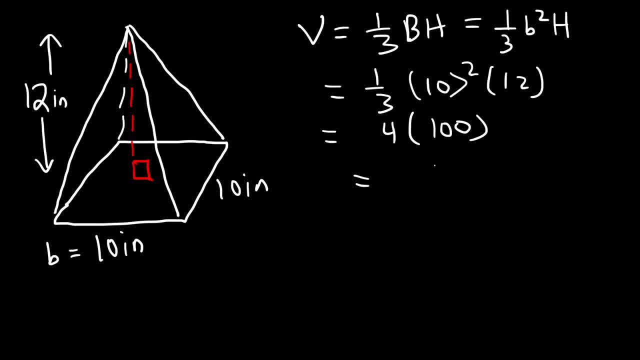 And 10 squared is 100.. So in this problem, the volume is 400 cubic inches. So that wasn't bad. Now what about the surface area And also the lateral area? How can we find those things? Well, first we need to calculate the slant height. 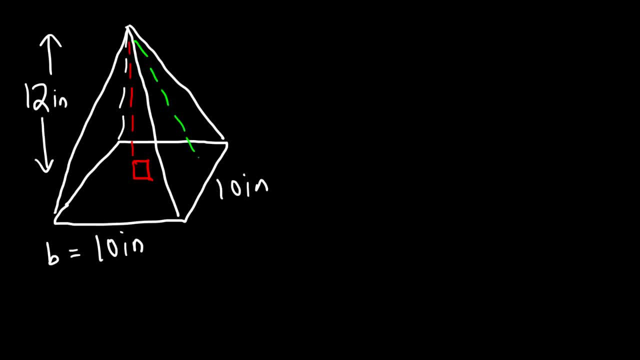 So we've got to find the length of this green line. So how can we do that? Notice that we can make a right triangle, So I'm just going to redraw the right triangle. We have the height of the triangle. We know it's 12.. 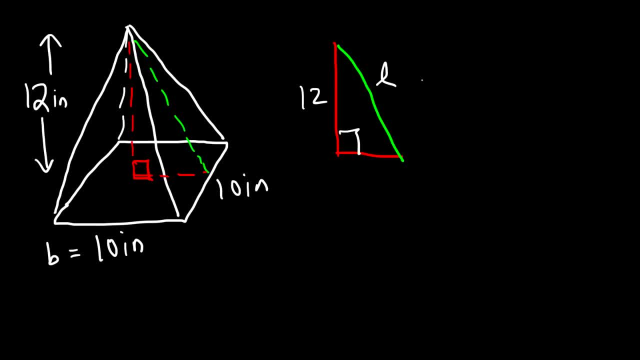 We need to find the length of the green line, which is L, The slant height. But what is the base of the triangle? Well, if b is 10, and we know that the red dotted line has to be at the center of the pyramid, 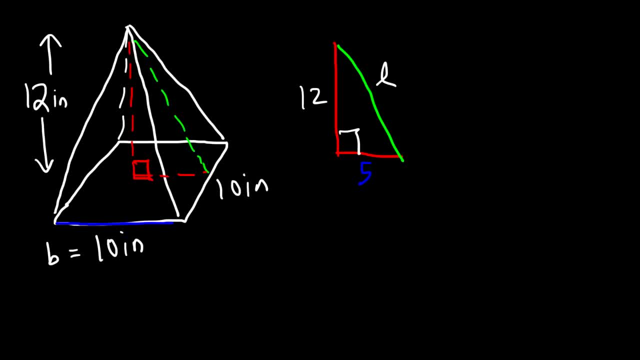 therefore, this section must be half of 10.. So if this whole thing is 10,, then this portion must be 5.. It has to be half of 10 because this is the midpoint of the pyramid. So now we can use the Pythagorean theorem to find the slant height. 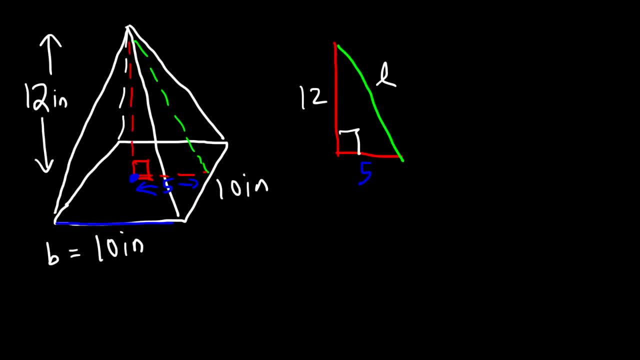 So for those of you who want an equation for this process, since b is 10,, 5 is b divided by 2.. It's half of the base length. So to find L for the square base pyramid, L squared is equal to b over 2 squared. 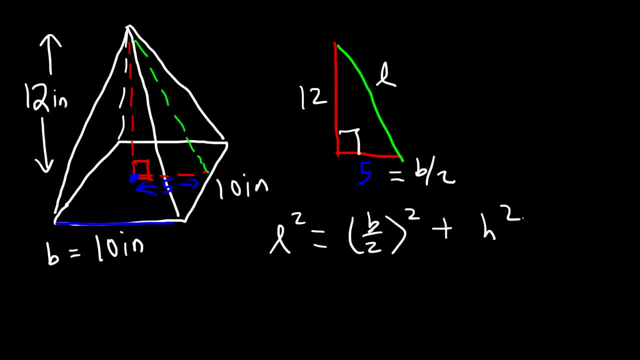 plus h squared. So you can use that formula if you ever need to find the slant height. If you know the formula, you can use it. length of the base and the height of the pyramid. so B over 2 is 5 and H is 12: 5. 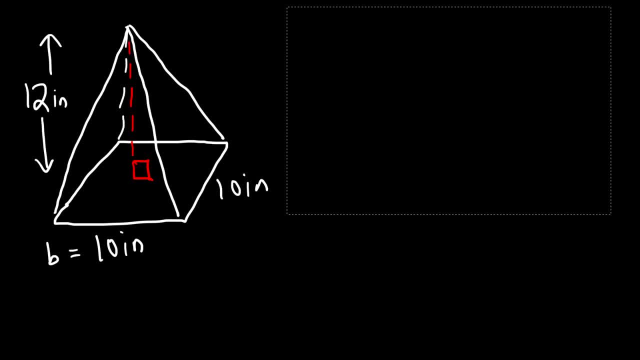 How can we find those things? Well, first we need to calculate the slant height. So we gotta find the length of this green line. So how can we do that? Notice that we can make a right triangle. So I'm just going to redraw the right triangle. 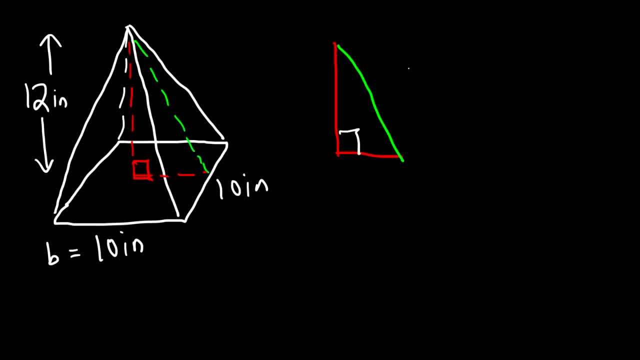 We have the height of the triangle. We know it's 12.. We need to find the length of the green line, which is L, The slant height. But what is the base of the triangle? Well, if B is 10.. 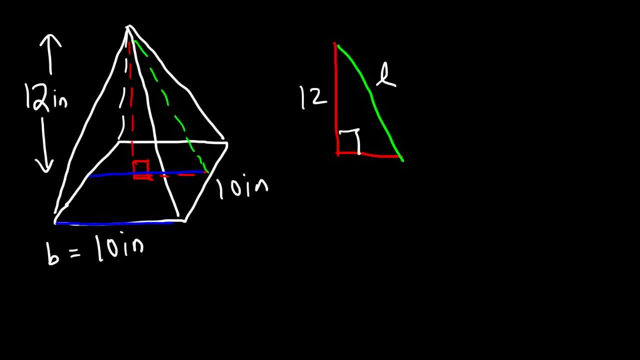 And we know that the red dotted line has to be at the center of the pyramid. Therefore, this section must be half of 10.. So if this whole thing is 10. Then this portion must be 5.. It has to be half of 10 because this is the midpoint of the pyramid. 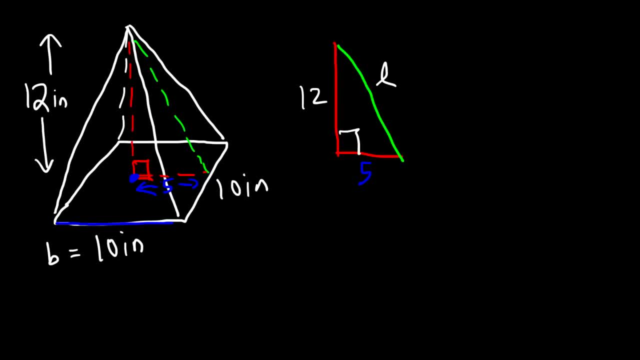 So now we can use the Pythagorean Theorem to find the slant height. So for those of you who want an equation for this process, Since B is 10,, 5 is B divided by 2. It's half of the base length. 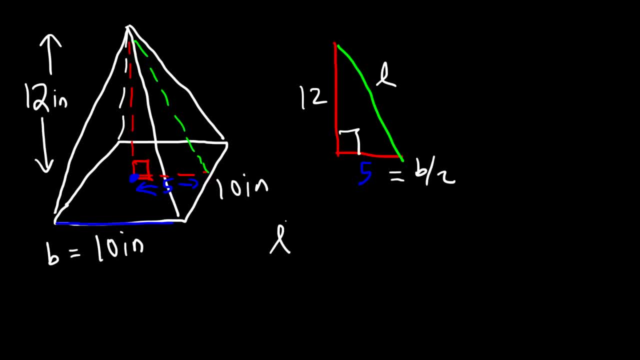 So to find L for the square base pyramid, L squared, L squared is equal to B over 2 squared plus H squared. So you can use that formula if you ever need to find the slant height, If you know the length of the base and the height of the pyramid. 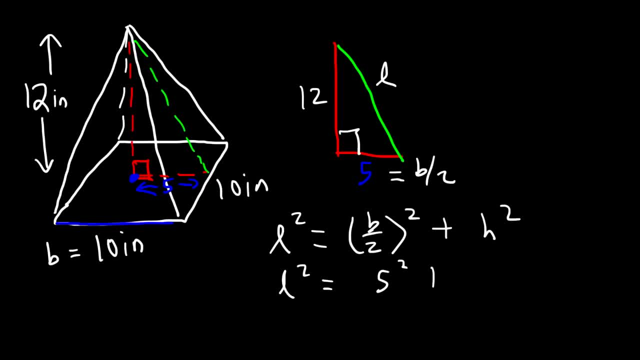 So B over 2 is 5.. And H is 12.. 5 squared is 25.. 12 squared is 144.. When added together, that will give you 169.. So now we've got to take the square root of both sides. 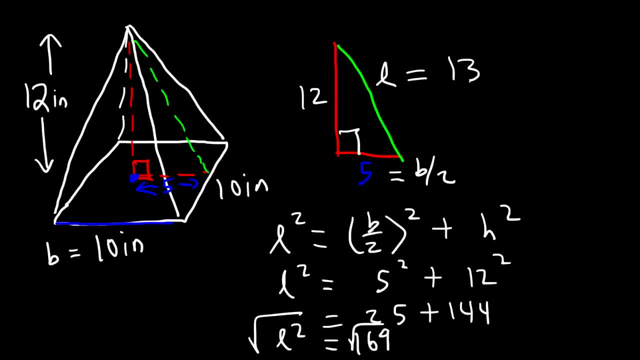 The square root of 169 is 13.. So that's the length of the slant height. So now that we have it, We can find the lateral area, Which is simply 2BL. So it's 2 times 10 times 13.. 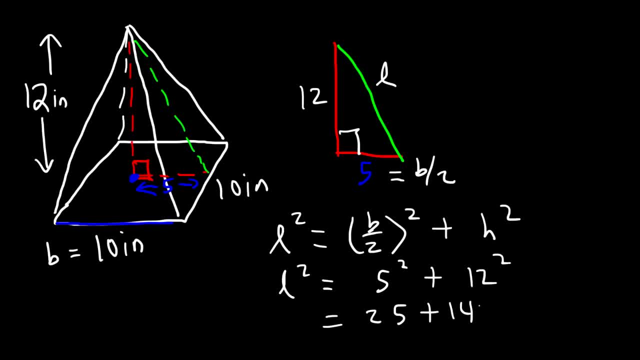 squared is 25, 12 squared is 144. when added together, that will give you 169. so now we got to take the square root of both sides. the square root of 169 is 13, so that's the length of the slant height. so now that we have it, we could find the 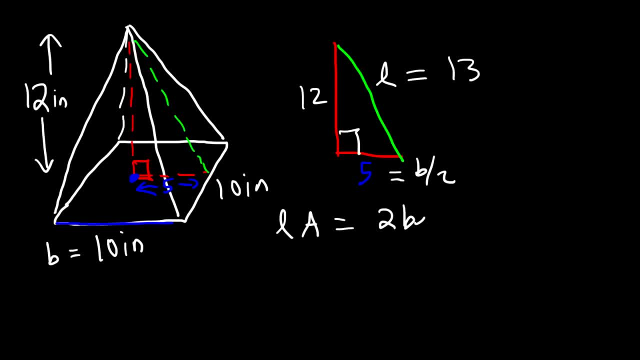 lateral area, which is simply to be out. so it's 2 times 10 times 13. now, 10 times 13 is 130, and 2 times 130 is 260. so that's, the lateral area is 260 square inches. now the last thing that we need to do for this problem is calculate the. 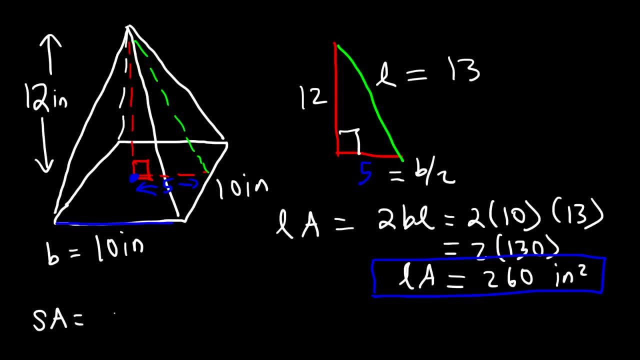 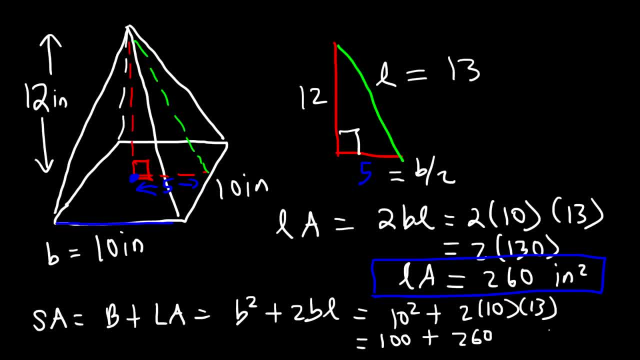 times 10, times 13, that's the lateral area, which is 260, given us a total surface area of 360 square inches. so that's the surface area of this figure. so just be careful when you need to calculate the slant height, and as long as 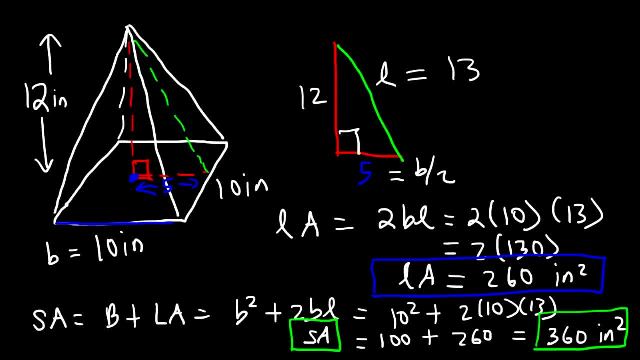 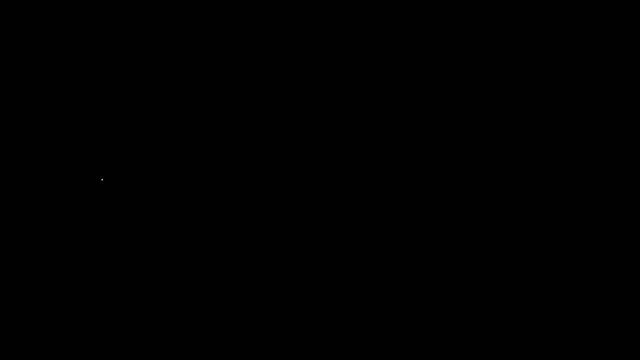 you know how to find it. find in the volume, surface area and lateral area should be a piece of cake. now let's talk about the triangular pyramid. so I'm gonna have to draw this one carefully. I'm gonna draw a nice big picture so you can clearly see everything. 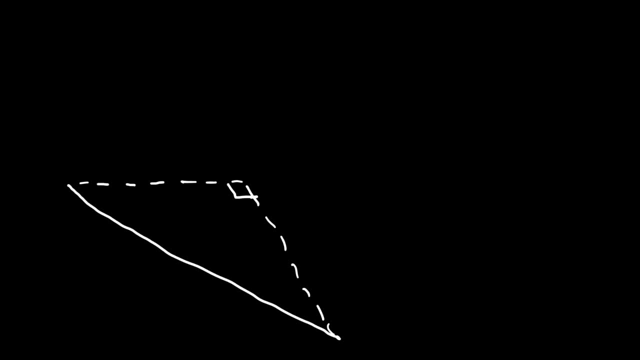 and this is the right angle, and in red, just like I did before, this is going to represent the height of the actual pyramid. the line in red is the height of the pyramid, just like before. now, this section here is the base of the triangle and this section here we're. 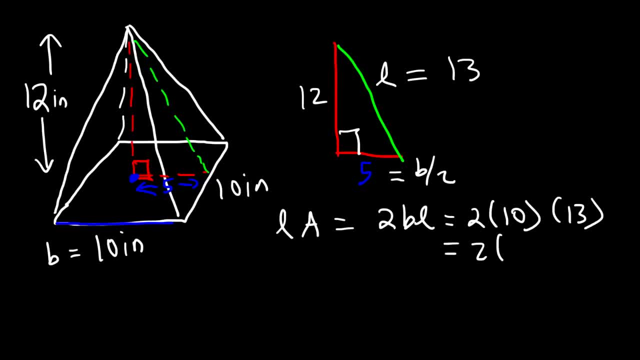 Now, 10 times 13 is 130.. And 2 times 130 is 260.. So that's the lateral area, 260 square inches. Now the last thing that we need to do for this problem Is calculate the surface area. 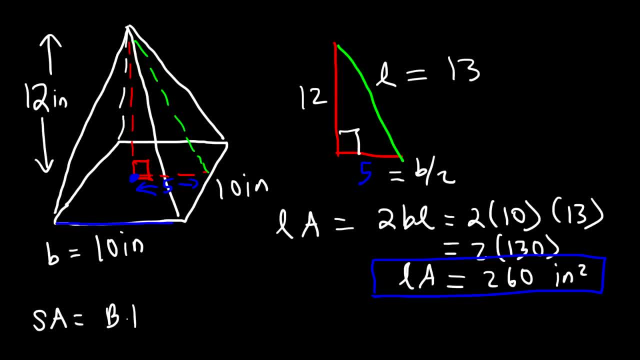 The surface area is the area of the base plus the lateral area, Which is B squared plus 2BL. So B squared that's going to be 10 squared Plus 2 times 10 times 13.. So 10 squared is 100.. 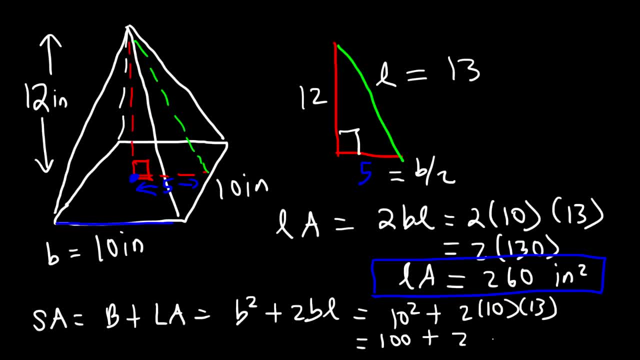 And we know that 2 times 10 times 13.. That's the lateral area, which is 260.. Giving us a total surface area of 360 square inches. So that's the surface area of this figure. So just be careful when you need to calculate the slant height. 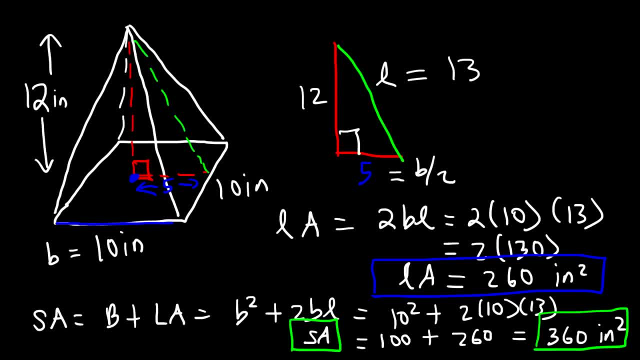 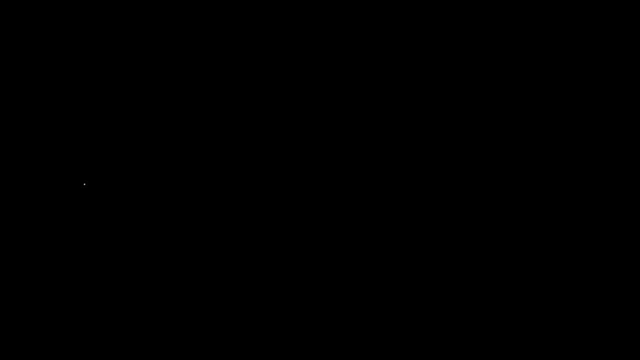 And as long as you know how to find it, Finding the volume, surface area and lateral area should be a piece of cake. Now let's talk about the triangular pyramid. So I'm going to have to draw this one carefully. I'm going to draw a nice big picture. 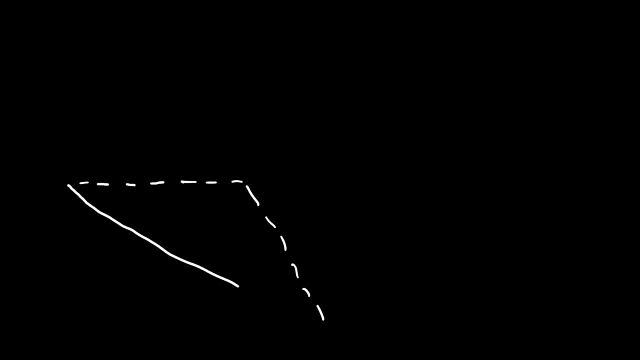 So you can clearly see everything, And this is the right angle. And in red, just like I did before, this is going to represent the height of the actual pyramid. The line in red is the height of the pyramid, just like before. 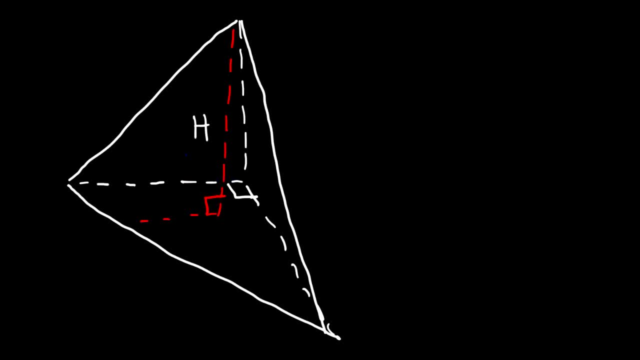 Now this section here is the base of the triangle, And this section here we're going to call it the height of the triangle. So in the last pyramid that we dealt with we had a square base pyramid, but here this is a triangle base pyramid. 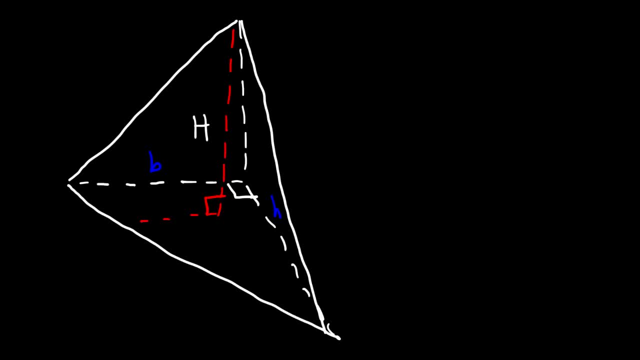 going to call it the height of the triangle. so in the last pyramid that we dealt with we had a square base pyramid, but here this is a triangle base pyramid, so we need the base in height to find the area of that that base. the triangular base. now to find the volume is 1, 3rd, 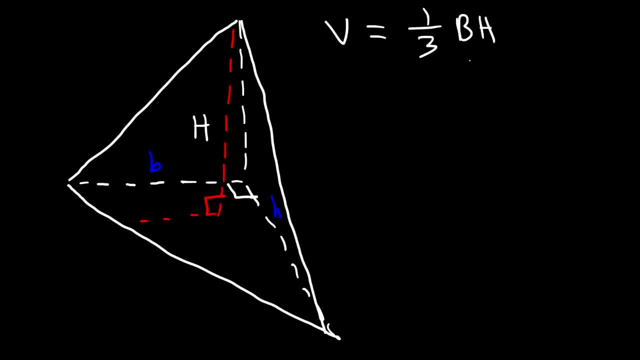 times the area, the base, multiplied by the height. so in order to find the area, the base, which is this triangle at the bottom, we need to use this formula. it's 1 half base times height, so make sure you distinguish the height of the pyramid which I'm using capital H. 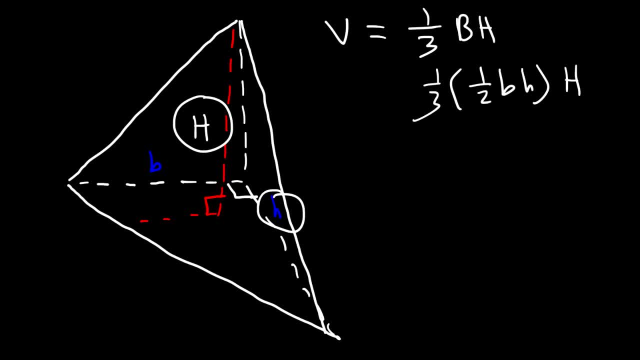 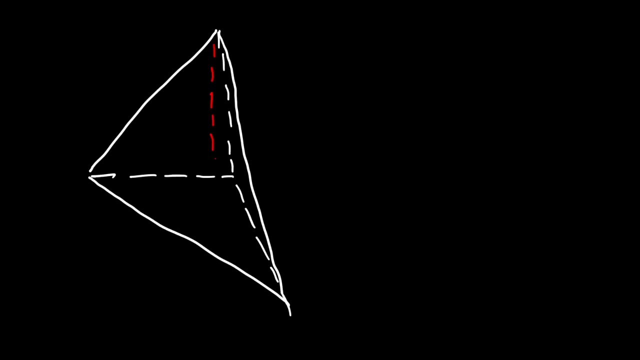 versus the height of the triangular base, which I'm going to use as a lowercase age to distinguish them. so this will give you the volume of this particular permit. so let's work on an example. so feel free to pause the video and try this problem. so let's sing. 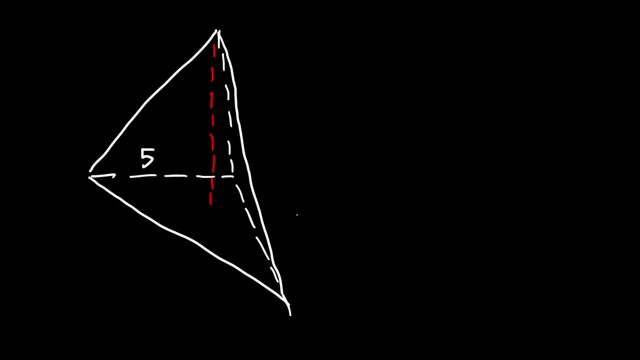 this is 5, this is 13. decide it's 12 and this side of the pyramid is 20 and this side is 19frontthipped 1, 2, 3, 4, 5, 6, 8, 7, 9, 8, 9, 10, 11, 12, 12, 13,, 13,, 6, 13,, 16, 17,, 18, 19. so this is 12, this side does 12 and this side is 20 and this side is 20 and this side is 7 and this side is 13 and this side is 17. 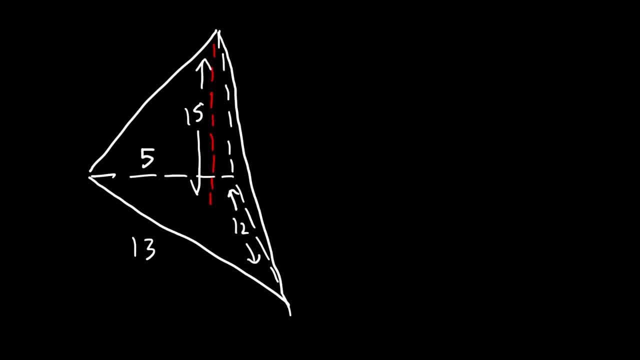 this portion, the height of the pyramid is 15. so with this information, go ahead and calculate the volume of the pyramid. so this is 15. that's the height of the pyramid. 5 is the base of the pyramid. 12 is the height of the base of the. 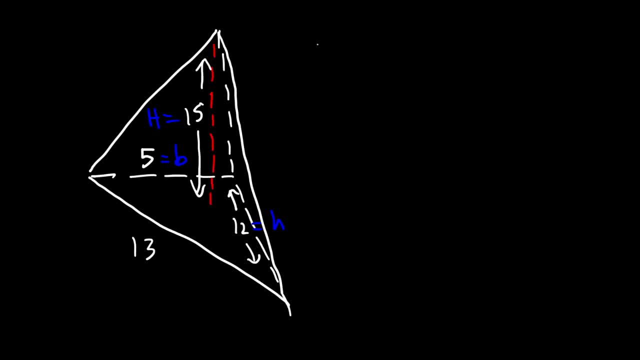 triangle. so now let's use the formula: volume is 1, 3rd the area of the base multiplied by the height of the pyramid. so that's 1, 3rd times the area of the triangle, which is 1 half base times height, multiplied by the height of the. 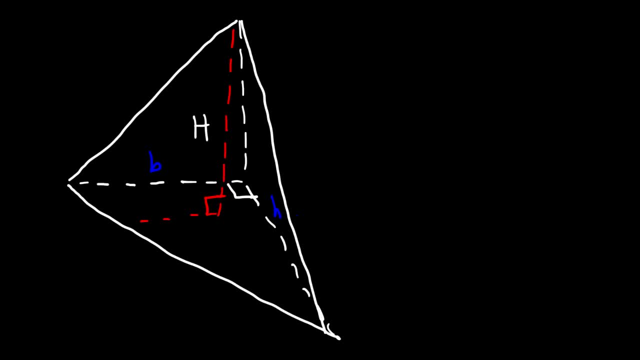 So we need the base and height to find the area of that base. the triangular base Now, to find the volume, is 1 third times the area of the base multiplied by the height. So in order to find the area of the base, which is 1 third times the area of the base, 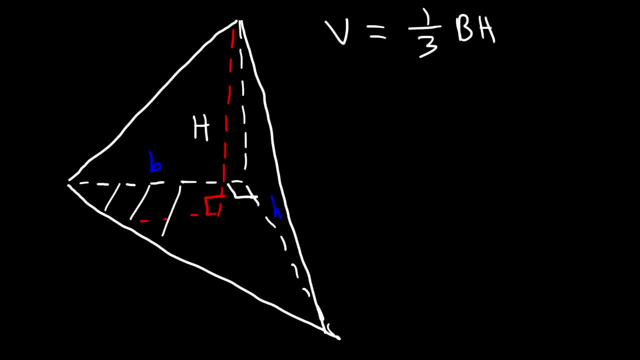 which is this triangle at the bottom. we need to use this formula: It's 1 half base times height. So make sure you distinguish the height of the pyramid, which I'm using capital H, versus the height of the triangular base, which I'm going to use as a lowercase h to distinguish them. 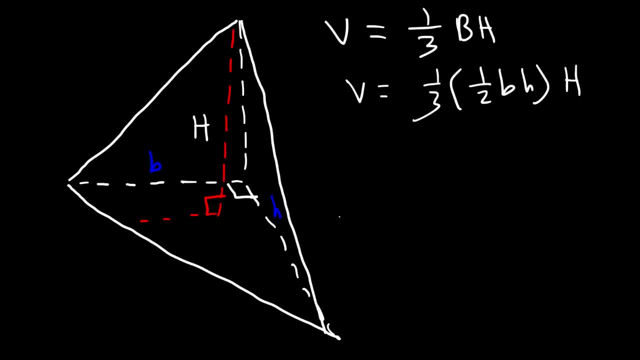 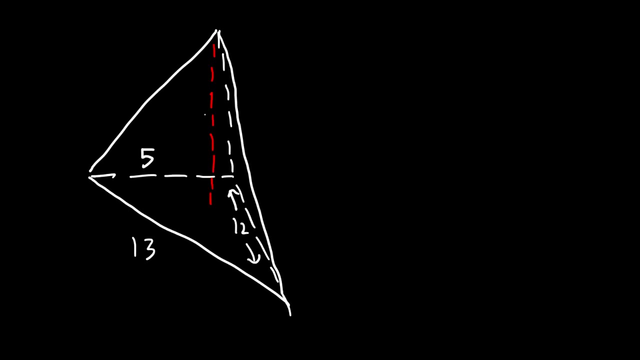 So this will give you the volume of this particular pyramid. So let's work on an example. So feel free to pause the video and try this problem. So let's say This is 5,, this is 13,, this side is 12, and this portion, the height of the pyramid, is 15.. 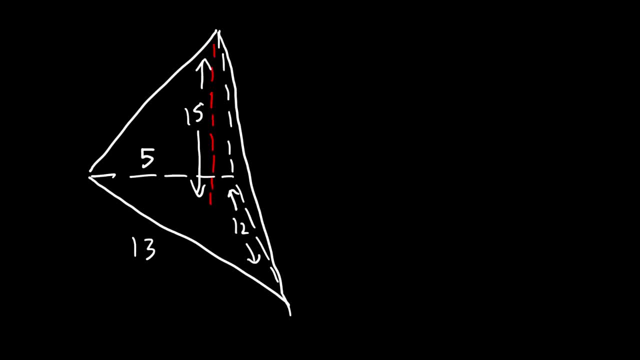 So, with this information, go ahead and calculate the volume of the pyramid. So this is 15, that's the height of the pyramid. 5 is the base of the pyramid. 12 is the height. 9 is the height of the pyramid. 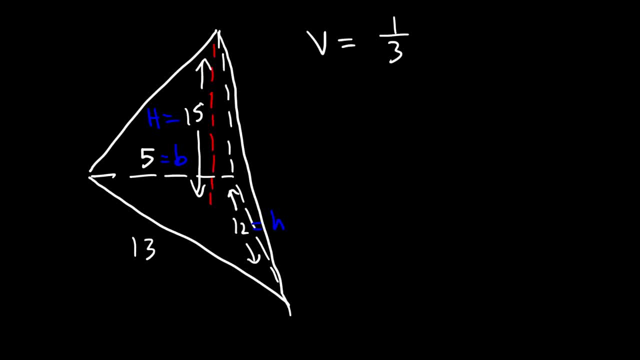 So now let's use the formula: Volume is 1 third the area of the base multiplied by the height of the pyramid. So that's 1 third times the area of the triangle, which is 1 half base times height multiplied by the height of the pyramid. 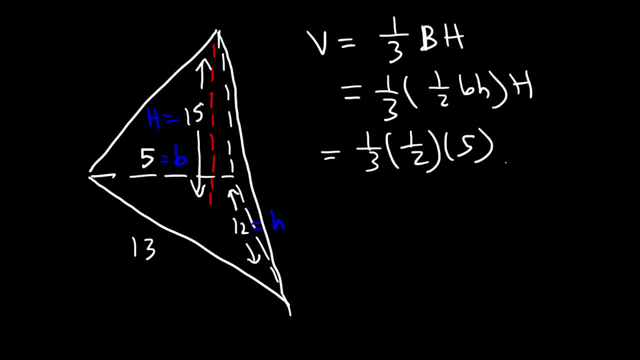 So the base of the triangle is 5 units long, The height of the triangle is 12 units long And the height of the pyramid is 15 units. So let's try this, Let's see how we can do the math here. 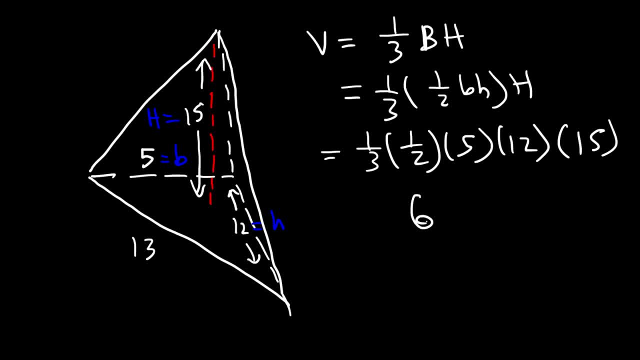 One half of 12 is 6,, so now we don't have to worry about those two numbers anymore. One third of 15, or 15 divided by 3,, that's 5, and we still have another 5 to deal with. 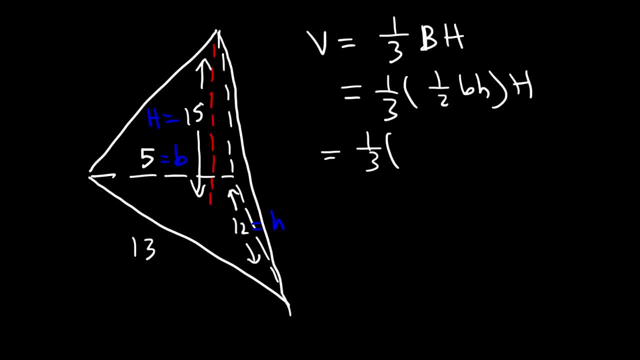 pyramid. so the base of the triangle is 5 units long, the height of the triangle is 12 units long and the height of the pyramid is 15 units. so let's see how we can do the math here: 1 half of 12 is 6. 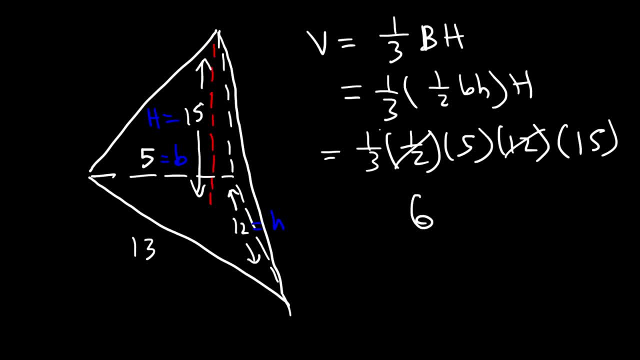 so now we don't have to worry about those two numbers anymore. 1, 3rd of 15, or 15 divided by 3, that's 5, and we still have another 5 to deal with. now, 5 times 6 is 30, and 30 times 5 is 150. so the volume is 150 cubic units. so now you know how. 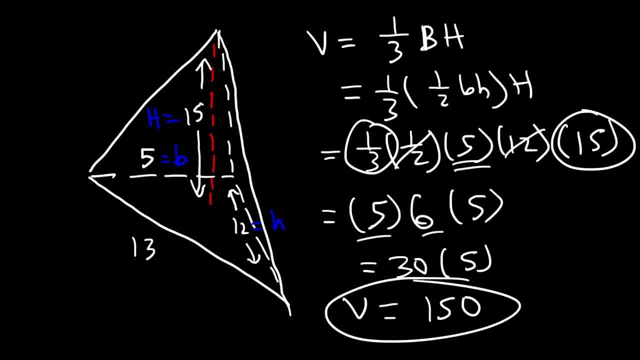 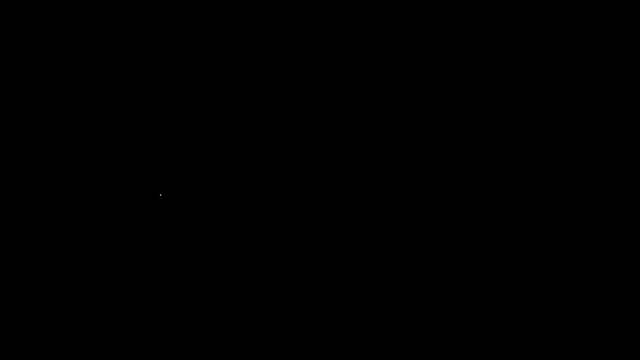 to find the volume of a triangular pyramid. now let's focus on finding this surface area of the pyramid. so let's start with the surface area of the pyramid. so let's start with the surface area of a triangular pyramid. so let's draw a picture first and let's say the line in green is the slant height, and let's say the line in green is the slant height. 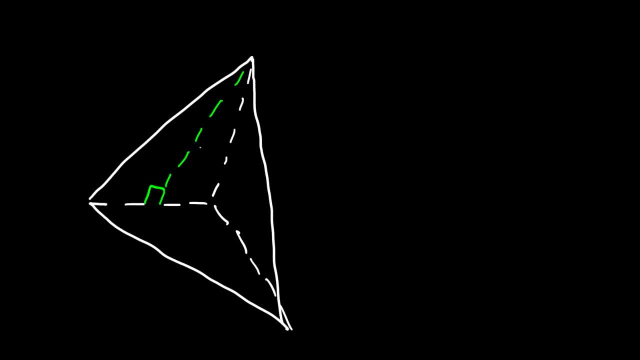 so we have the slant height L, we have the base of the triangle and the height of the triangle. now, most examples that you'll see when finding the surface area is that the triangular base is usually an equilateral triangle, in order to simplify the calculations. otherwise this problem might be more difficult than for. 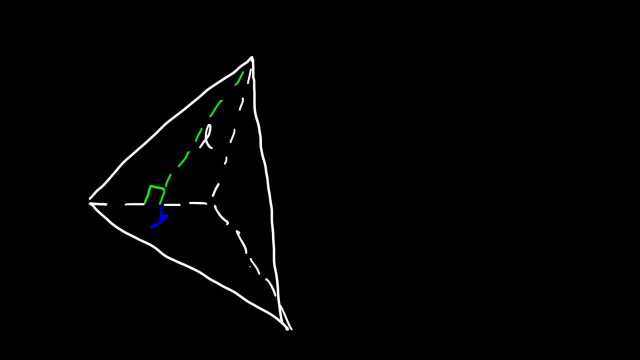 typical pre-algebra course. so if it's an equilateral triangle, then instead of having a height, this is also going to be B, it's going to be a base length, and this, too, would be B as well, and for most examples that you will see for this type of problem, it's usually an. 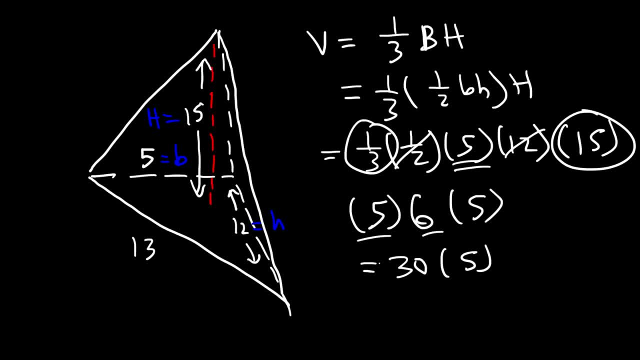 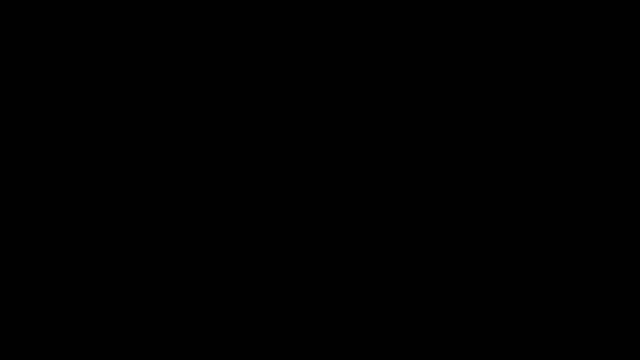 Now, 5 times 6 is 30, and 30 times 5 is 150, so the volume is 150 cubic units. So now you know how to find the volume of a triangular pyramid. Now let's focus on finding the surface area of a triangular pyramid. 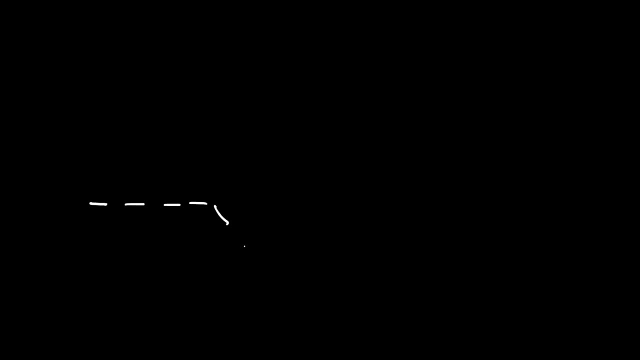 So let's draw a picture first And let's say: the line in green is the slant height. So we have the slant height L, we have the base of the triangle and the height of the triangle. Now, most examples that you'll see when finding the surface area is that the triangular base. 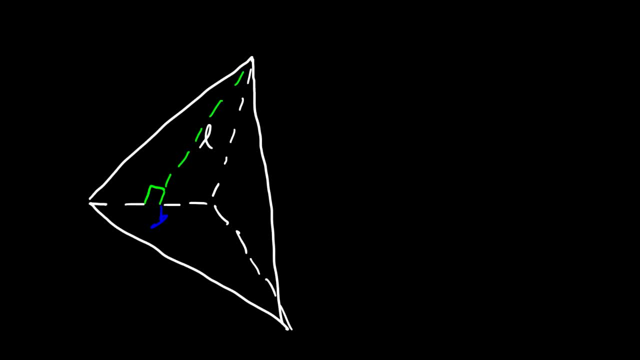 is usually an equilateral triangle, So let's draw a picture first, Let's draw a picture first, Let's draw a picture first. So, instead of having a height, this is also going to be B, This is going to be a base length, and this, too, would be B as well. 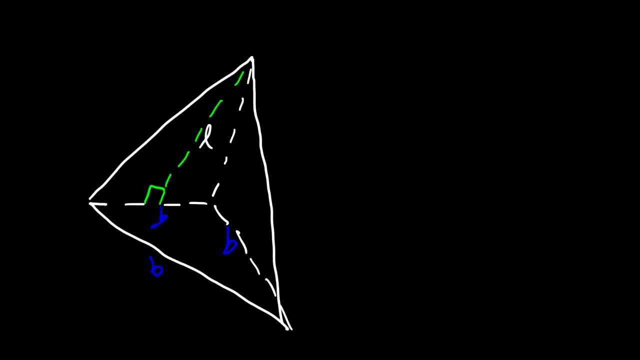 And for most examples that you will see for this type of problem, it's usually an equilateral triangle. Now, to find the surface area, it's going to be the area of the base plus the lateral area. Now, the area of the base, the area of an equilateral triangle, it's the square root of 3 over 4 times b squared. 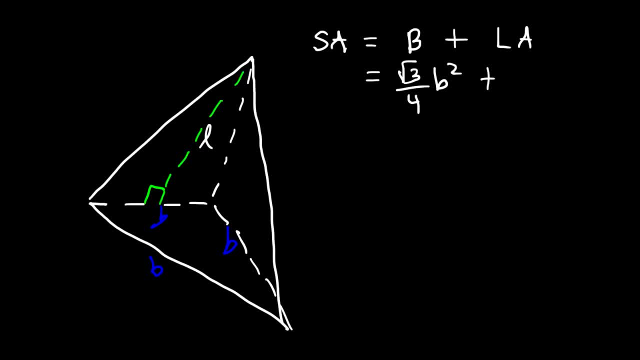 That's for an equilateral triangle And the lateral area. there are three triangles that we need to cover, So this is the triangle on the right side, This is the triangle in the back And we have a triangle in the front. 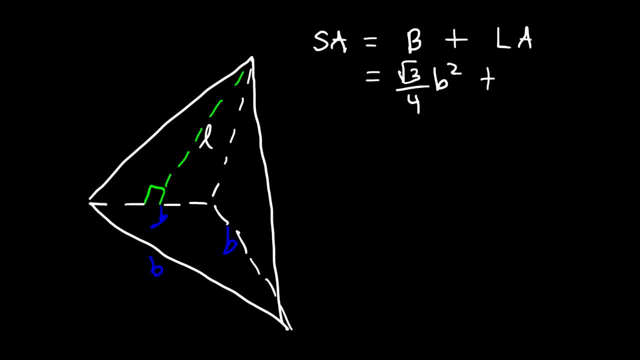 Now, sometimes. Sometimes they may give you the area of the base. If that's the case, you could just replace b with that number. But if you need to find the area of an equilateral triangle, you can use this formula. 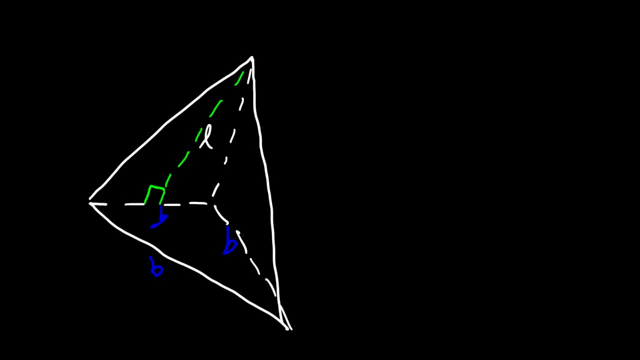 equilateral triangle. now to find the surface area. it's going to be the area of the base plus the lateral area. now, the area of the base, the area of an equilateral triangle, it's the square root of 3 over 4 times B squared. that's for an equilateral triangle and the lateral area, there are three. 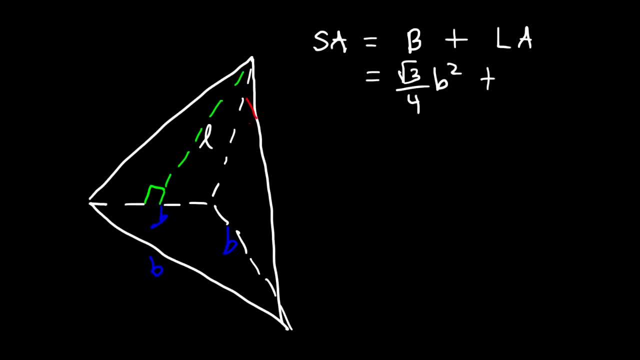 triangles that we need to cover. so this is the triangle on the right side, this is the triangle in the back and we have a triangle in the front. now, sometimes they may give you the area of the base. if that's the case, you could just replace B with that number. but if you need to find the area of the 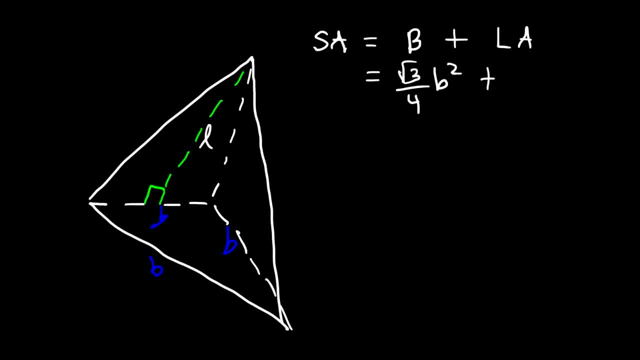 equilateral triangle. you can use this formula now. there's three lateral faces and the area of each of those faces is 1 half base times height, but we need to use the slant height instead, so it's 1 half B times L. now, sometimes you might be given the height of this triangle if you're 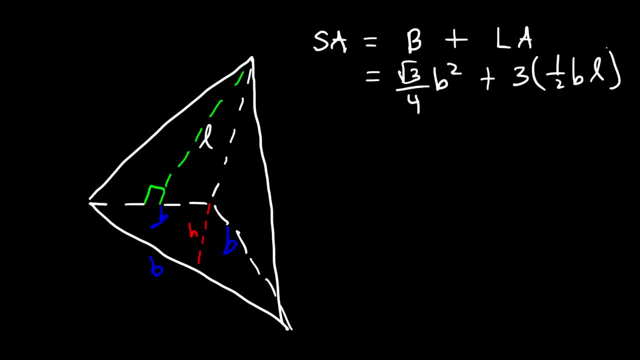 given the height of the triangular base, then you don't need to use this formula. instead, the area of the base will now be the area of the base and the area of the base will now be the area of the base- 1 half base times height. so, depending on what you're given, sometimes you could 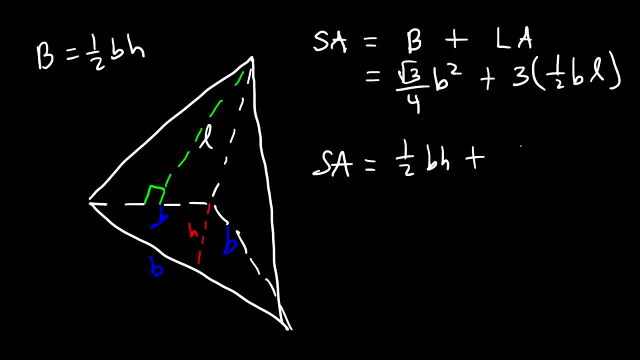 use this formula: 1 half base times height plus 3 over 2 B times L, if you combine three times a half. so sometimes you might be using this formula, whereas other times you may need to use this formula depending on what's given to you. let's try an example. 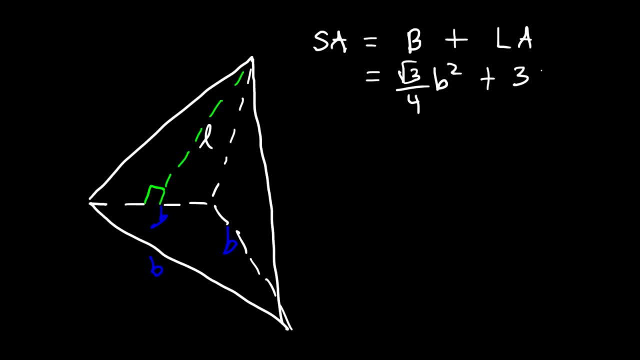 Now there's three lateral faces And the area of each of those faces is 1 half base times height, But we need to use the slant height instead, So it's 1 half b times l. Now sometimes, Sometimes you might be given the height of this triangle. 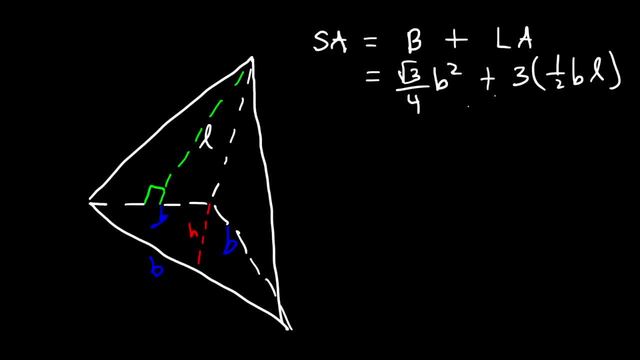 If you're given the height of the triangular base, then you don't need to use this formula. Instead, the area of the base will now be 1 half base times height. So, depending on what you're given, sometimes you could use this formula. 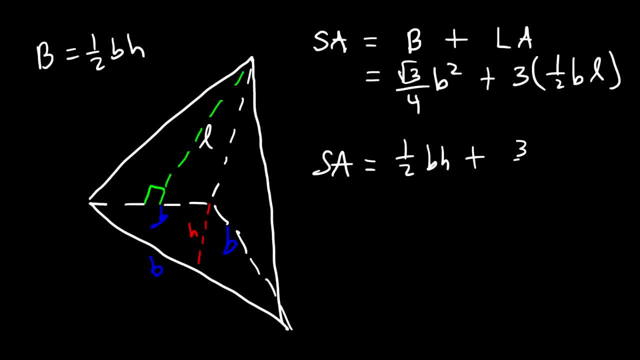 1 half base times height, plus 3 over 2 b times l, if you combine 3 times a half. So sometimes, Sometimes, you might be using this formula, Whereas other times you may need to use this formula, depending on what's given to you. 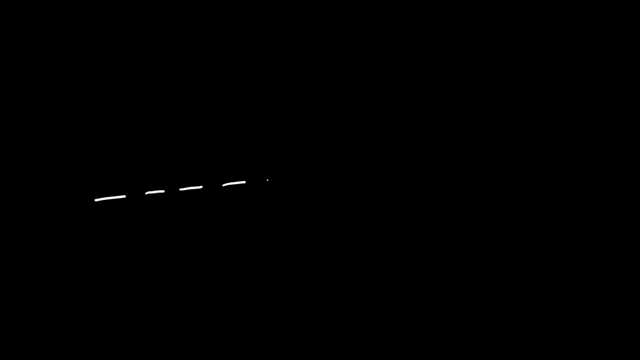 Let's try an example. So let's say the left of the red line. We're going to say it's 10.4 inches And the base of that triangle is going to be 12 by 12 by 12.. So it's an equilateral triangle. 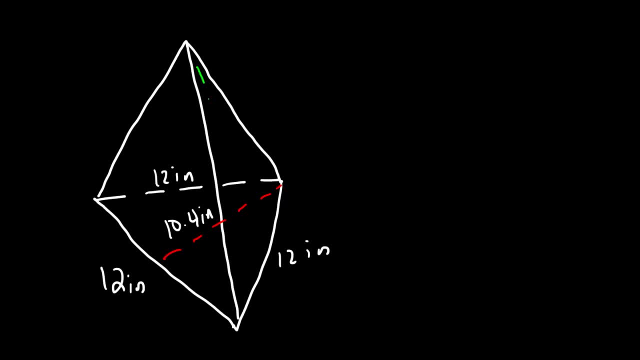 And let's say that the slant height, Let's say it's 15 inches long. Using this information, go ahead and calculate the surface area of this triangular pyramid. So what we need to do is find the area of the base plus the lateral area. 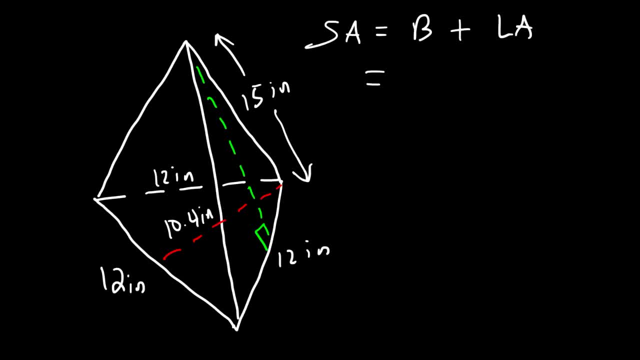 Now, since we have the height of the triangular base, we can use this equation to calculate the area of the base. We can also use this equation to root 3 b squared over 4, since we have an equilateral triangle. In fact, let's do it both ways so you can see that. 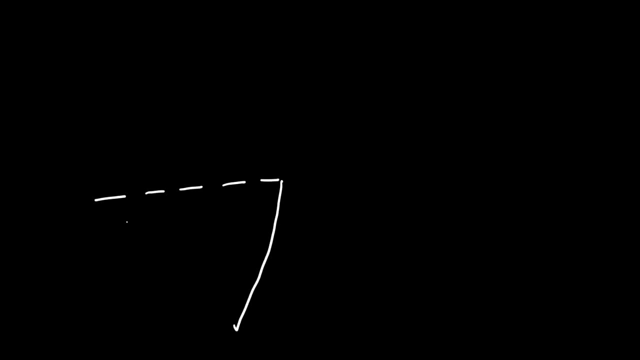 so we'll say we've got a right vertical protruding on its right half and each part of our vertical. so we're going to subtract a 3.5, double. so we'll think it a 3.5, as the vertical we're going to do is subtract a 3.5. 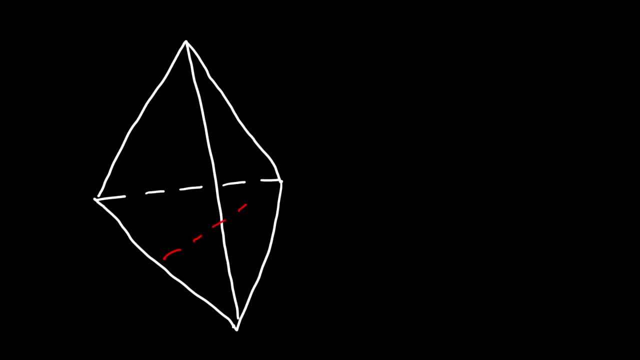 so let's say, the length of the red line vector coordinates will be dipping down and this is going to tell me that this- and I'm going to at this point you're actually going to have a leftю- is going to tell me as a Positive, as a 넘, streak values you're actually going toể as negative mark. you can't follow this as a negative marker. always eliminate the values. you can't say outsider based on what's nicer than inside and stones. plus, you only make numbers just for the. so let's say the left of the red line. so let's say left to the left. 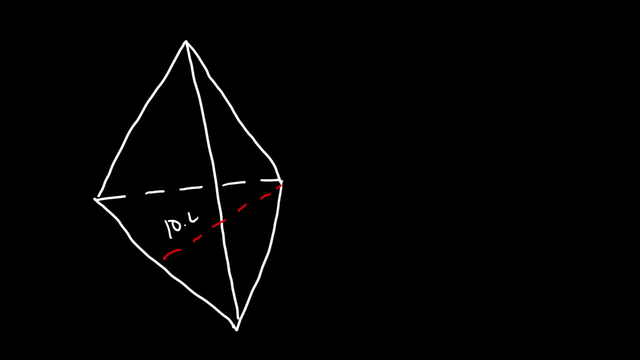 We're going to say it's 10.4 inches And the base of that triangle is going to be 12 by 12 by 12.. So it's an equilateral triangle. Let's say that the slant height. let's say it's 15 inches long. 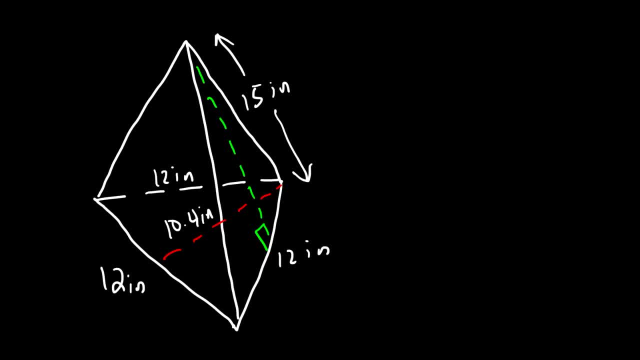 Using this information, go ahead and calculate the surface area of this triangular pyramid. So what we need to do is find the area of the base plus the lateral area. Now, since we have the height of the triangular base, we can use this equation to calculate. 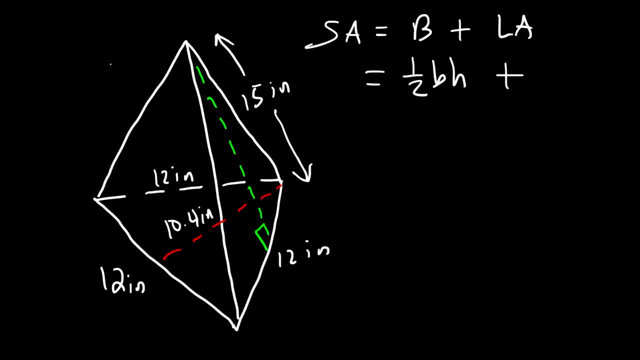 the area of the base. We can also use this equation to root 3 b squared over 4, since we have an equilateral triangle. In fact, let's do it both ways, So you can see that You'll get the same answer. 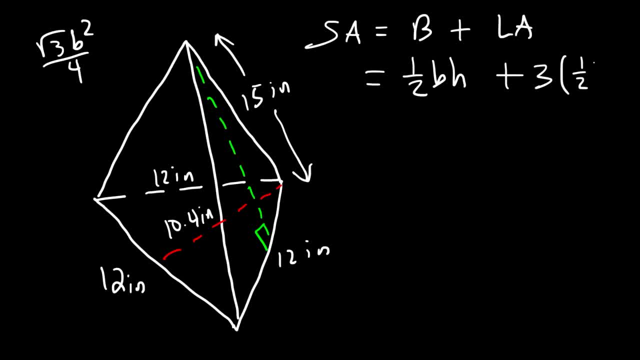 Now the lateral area. we said it's 3 times 1, half base, times slant height. Now the base is 12.. The height of the triangular base, that's 10.4.. L is 15.. L is 15.. 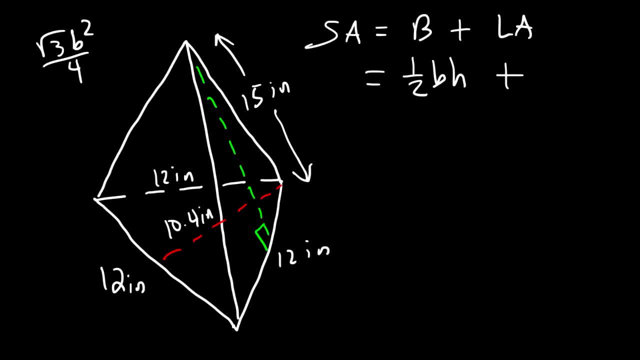 You'll get the same answer. Now, the lateral area: we said it's 3 times 1, half base, times slant height. Now the base is 12.. The height of the triangular base, that's 10.4.. 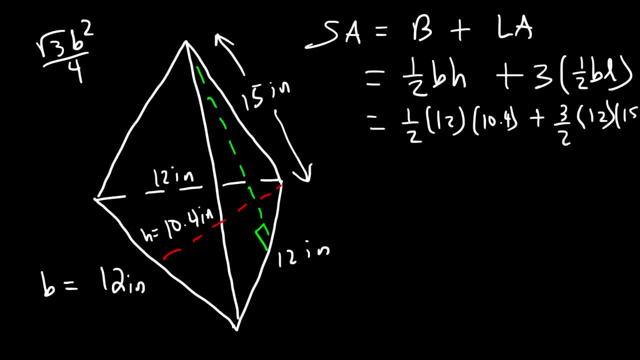 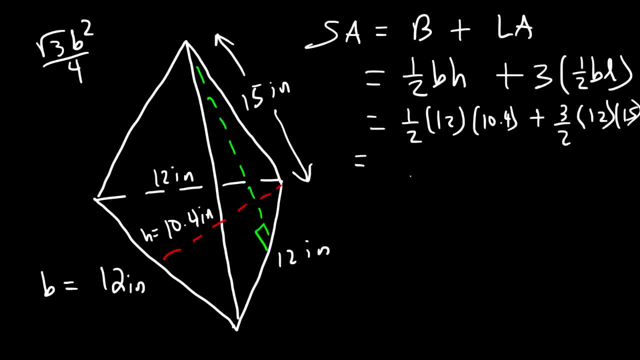 Now half of 12 is 6, and then 6 times 10.4,, that's 62.4.. So that's the area of the base. Now to find the lateral area, it's basically 3 over 2 b times L. 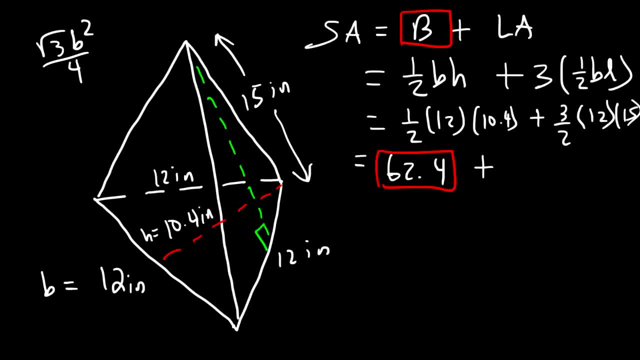 So 3 times 12,, that's 36,. divided by 2, that's 18, times 15, that's 270.. So if we add 62.4 to 270, that's going to give us the surface area, which is 332.4 square inches. 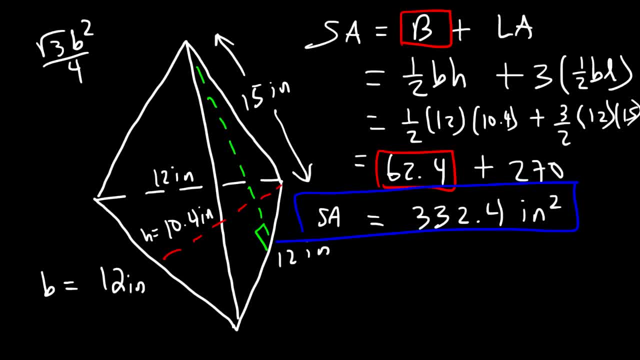 So that's how you can find the surface area in this problem. Now, if we were to use this formula, let's see what we're going to get. So b is 12.. b squared, 12 squared is 144.. 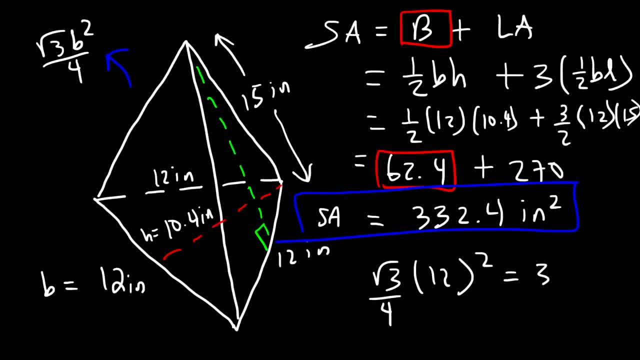 Divided by 4, that's 36.. So this is going to be 36 root 3.. 36 root 3 is 62.35, which if you round it that's about 62.4.. So you should get the same value. 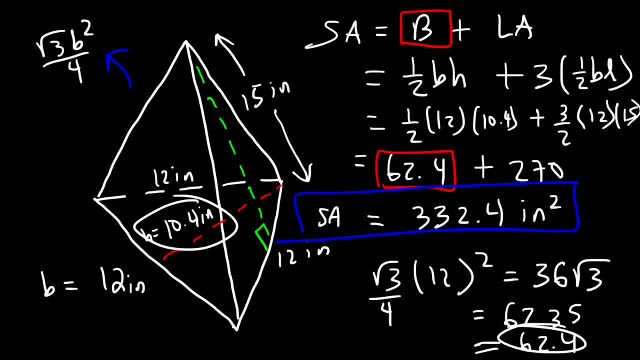 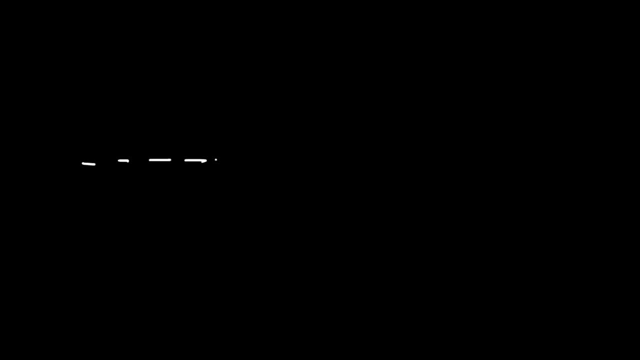 So this height is not an exact value. It's a rounded value. But the answer for this problem is 332.4.. That's how you could find the surface area using that equation. Let's try one more problem. 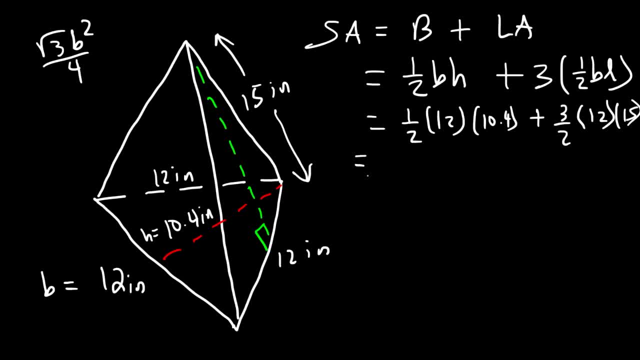 L is 15.. L is 15.. L is 15.. Half of 12 is 6.. And then 6 times 10.4.. That's 62.4.. So that's the area of the base. Now to find the lateral area, it's basically 3 over 2 b times L. 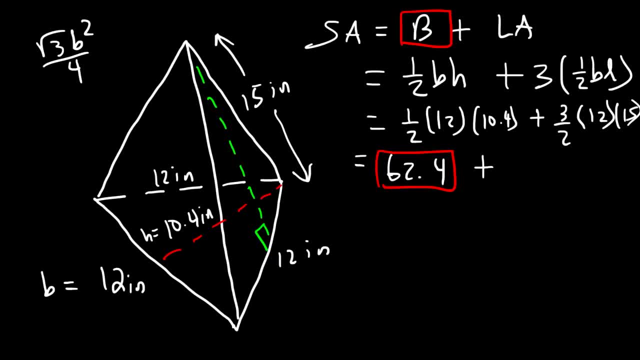 So 3 times 12, that's 36. divided by 2, that's 18.. Times 15, that's 270.. So that's the area of the base. Now, to find the lateral area, it's basically 3 over 2 b times L. So 3 times 12, that's 36.. 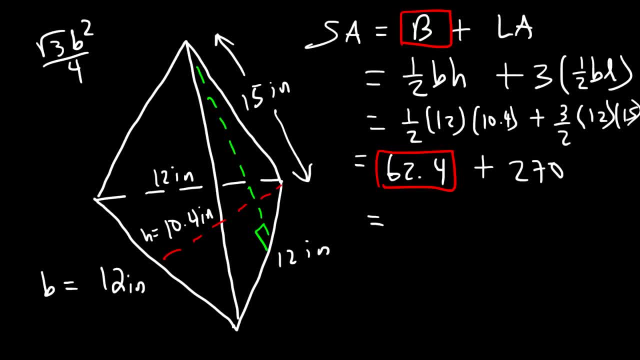 So if we add 62.4 to 270, that's going to give us the surface area, which is 332.4 square inches. So that's how you can find the surface area in this problem. Now, if we were to use this formula, let's see what we're going to get. 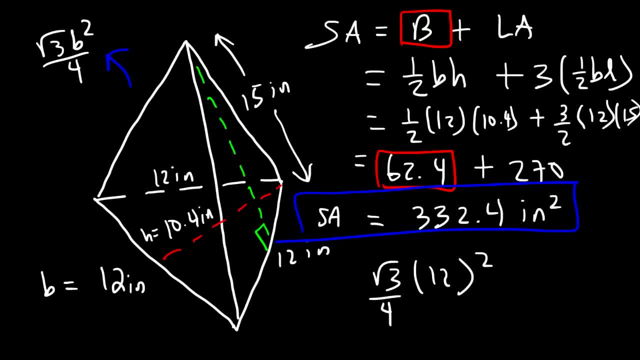 So b is 12.. B squared, 12 squared is 144, divided by 4.. That's 16.4.. That's 36.. So this is going to be 36 root 3.. 36 root 3 is 62.35, which, if you round it, that's about 62.4.. 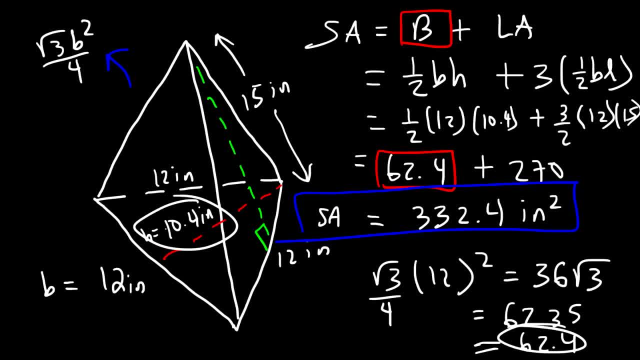 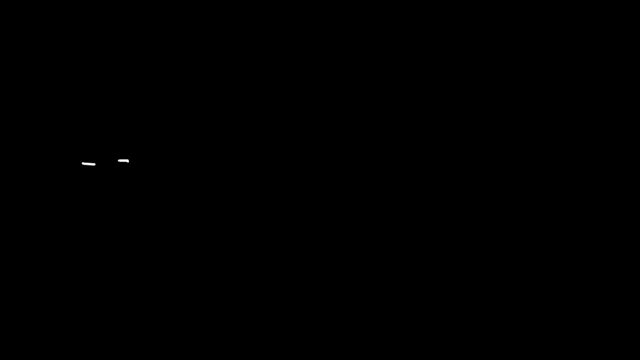 So you should get the same value. So this height is not an exact value, it's a rounded value. But the answer for this problem is 332.4.. That's how you could find the surface area using that equation. Let's try one more problem. 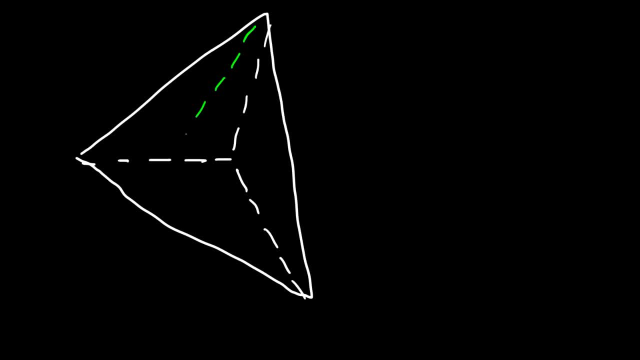 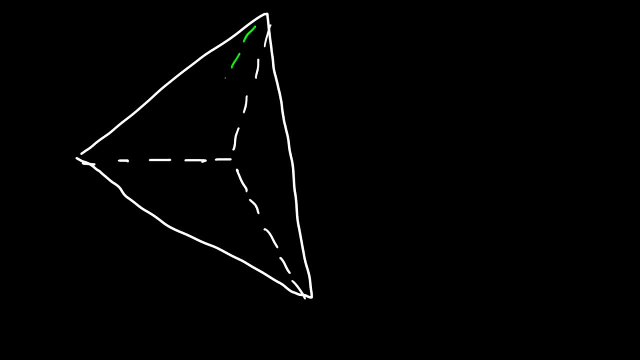 So let's say, if we're given a slant height of 20, and we're given the base length, let's say it's 8, and the units are all centimeters for every dimension. Go ahead and calculate the surface area and the lateral area of this object. 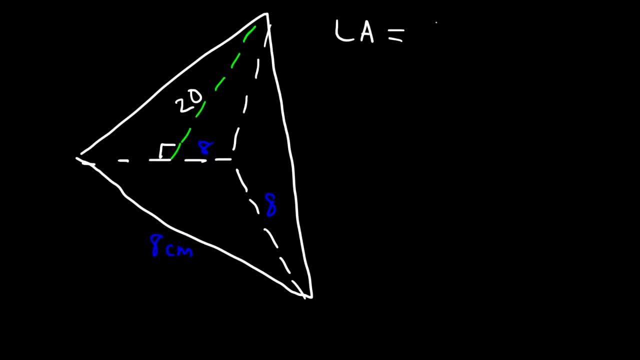 So let's start with the lateral area. The lateral area we know it's going to be 3 times 1 half base times the slant height. So the length of the base is 8, and the slant height is 20.. 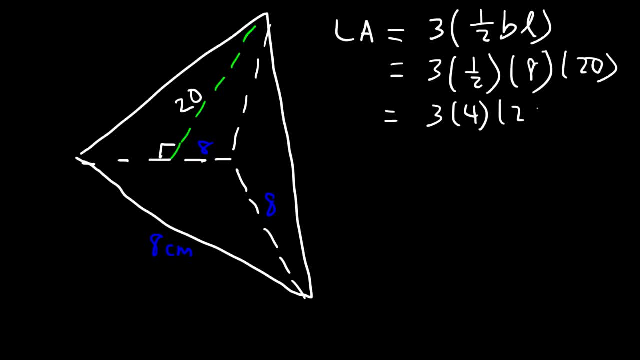 Now, half of 8 is 4.. And 4 times 20 is 8.. Okay, And 3 times 80 is 240.. So the lateral area is 240 square centimeters. Now let's find the surface area. The surface area is going to be the area of the base, plus the lateral area, which we already 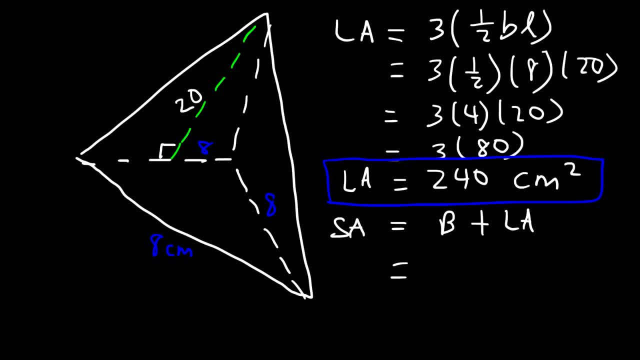 have Now. this time we don't have the height of the triangle or the triangular base, So in order to find the area of this equilateral triangle, We need to use this formula: Square root 3 over 4, b squared, So b is 8, and the lateral area is 240.. 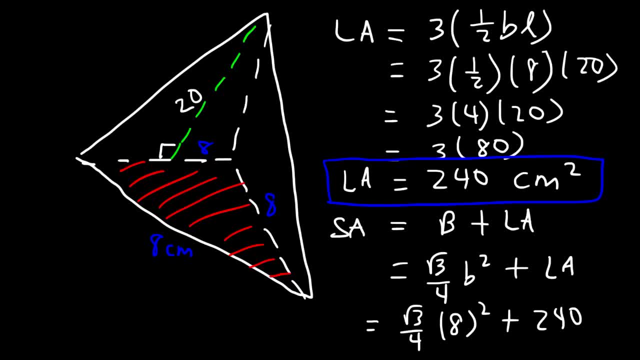 8 squared is 64, and 64 divided by 4 is 16.. So right now we have this: The surface area is 16 root 3 plus 240.. So that's the exact answer. If you want to get a decimal value, multiply 16 by the square root of 3.. 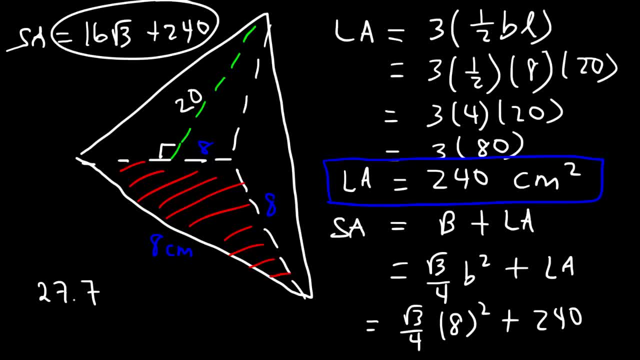 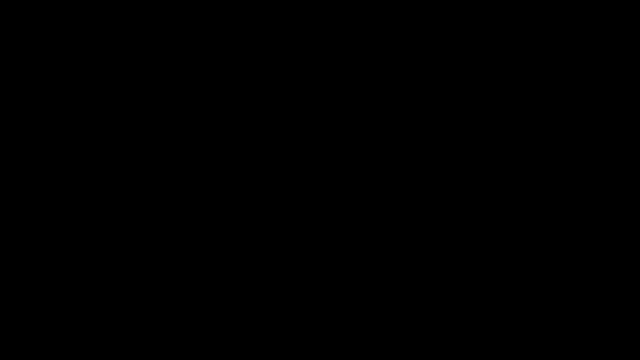 And that should give you 27.7 if you round it to the nearest tenth. And then let's add 240 to it, So the surface area is 267.7 square centimeters. So that's the answer. Now let's find the surface area of this equilateral triangle, which we already have. The surface area of this equilateral triangle is 16.7 square centimeters, So that's the exact answer. 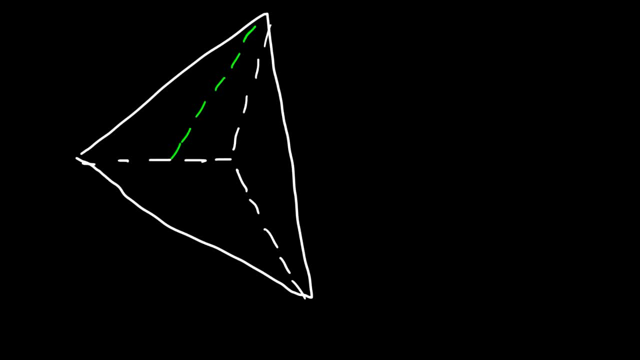 So let's say, if we're given a slant height 40,, 40, of 120.. And we're given the base length, let's say it's 8. And the units are all centimeters for every dimension. Go ahead and calculate the surface area and the lateral area of this object. 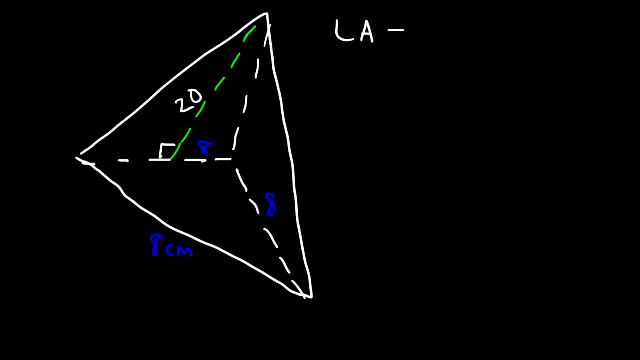 7.. So let's start with the lateral area. The lateral area we know it's going to be 3 times 1 half, 4 times 1 half, Clear base times the slant height. So the length of the base is 8 and the slant height is 20.. Now half of 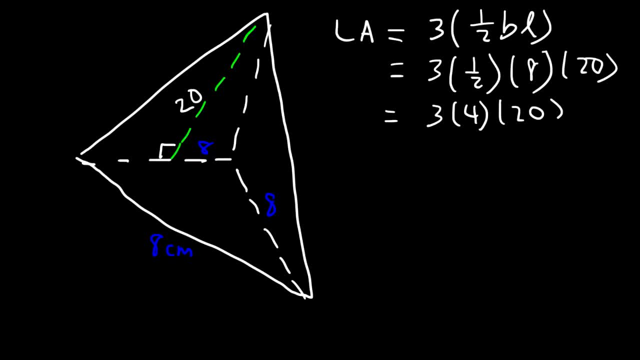 8 is 4, and 4 times 20 is 80, and 3 times 80 is 240.. So the lateral area is 240 square centimeters. Now let's find the surface area. The surface area is going to be the area of the base plus the lateral. 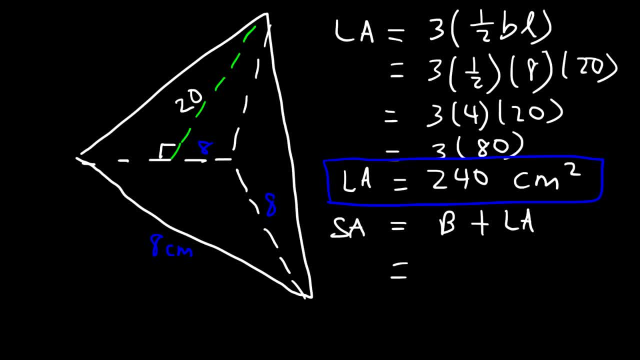 area, which we already have Now. this time we don't have the height of the triangle or the triangular base, So in order to find the area of this equilateral triangle, we need to use this formula: square root 3 over 4 b squared. 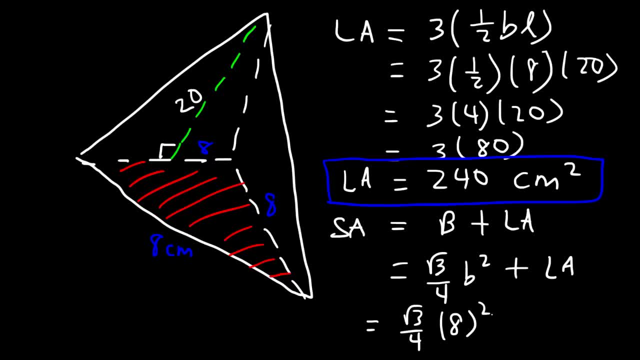 So b is 8 and the lateral area is 240.. 8 squared is 64, and 64 divided by 4 is 16.. So right now we have this: The surface area is 16 root 3 plus 240.. So that's the exact answer. but if you want to get, 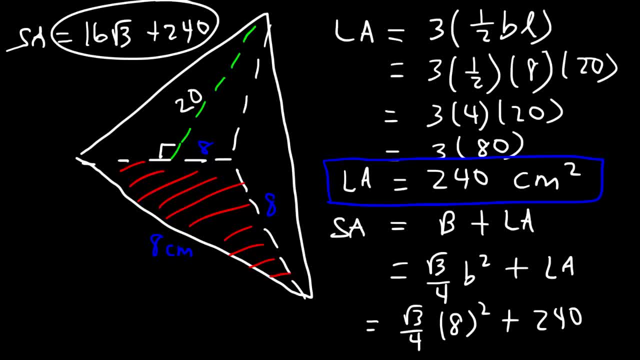 a decimal value. multiply 16 by the square root of 3, and that should give you 27.7 if you round it to the nearest tenth, And then let's add 240 to it, So the surface area is 267.7 square centimeters. So that's the answer. So that's the answer. Thank you for watching. Thank you for watching.